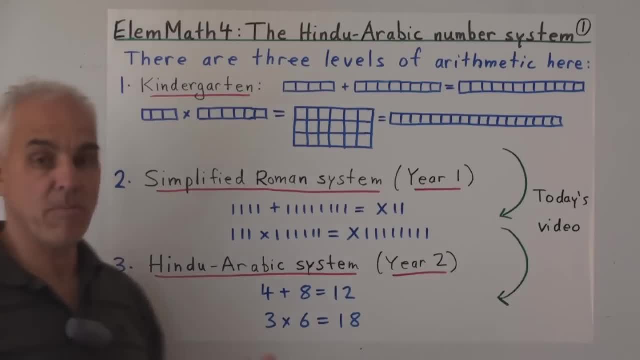 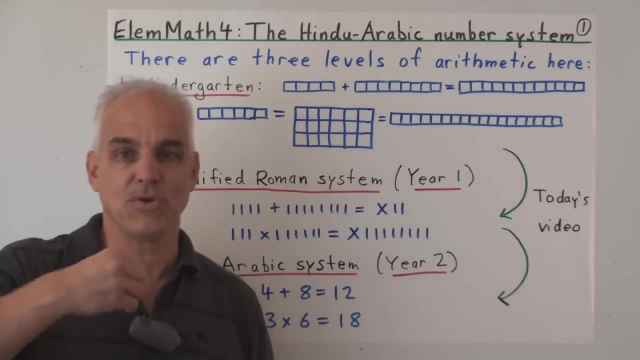 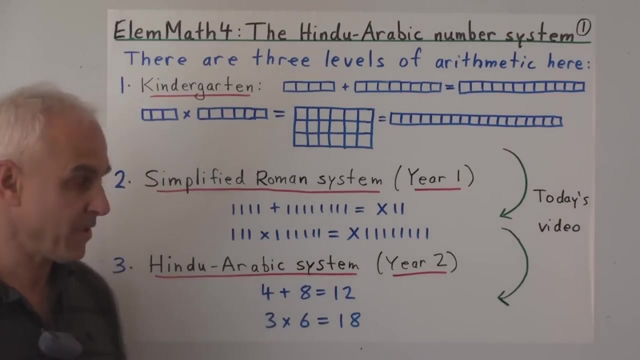 So I don't think that's really that important. What's more important is that they learn how to count, that they learn that numbers are something that one uses to count, And in fact, it's better for them not to learn that with the Hindu Arabic number system, but rather to learn it with this kindergarten approach that I've told you about, where the numbers are represented by rows of unit cells and where the arithmetic is particularly simple. 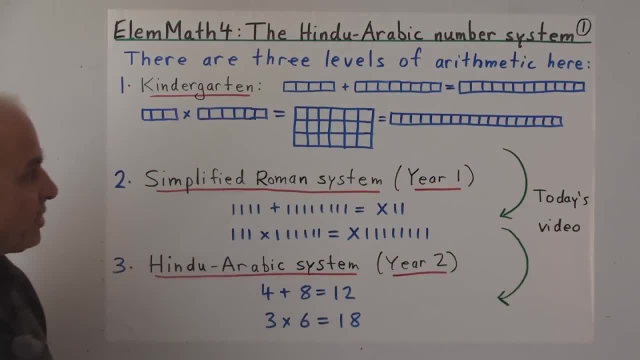 At least. addition is very simple. Just put rectangles together and multiplication is reasonably simple. Make a rectangle. Make a rectangle whose dimensions are the two numbers we're started with In this case, that one is there and that dimension is there- And then count the number of cells in that rectangle. 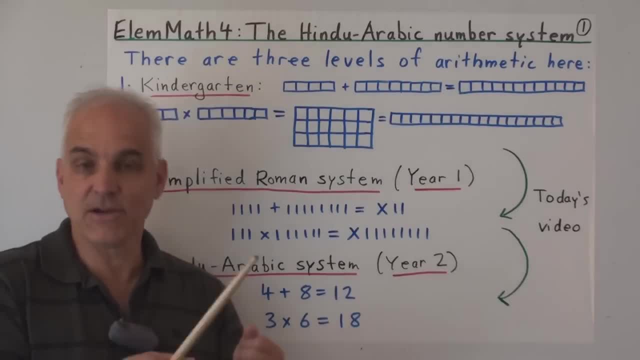 So these are very geometrical, almost physical things that young people can start out learning long before they're able to draw anything coherent on a page. So, for example, So, for example, there's a pleasant game called Blockus that involves little plastic pieces like this: 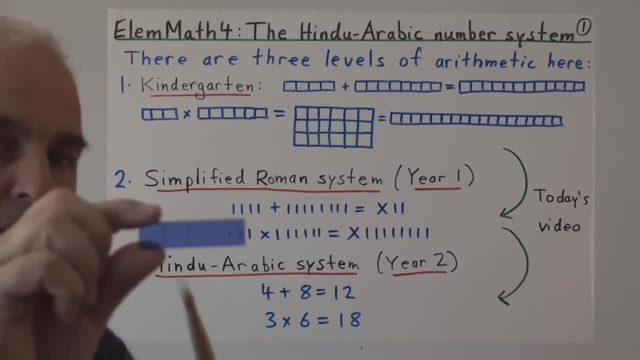 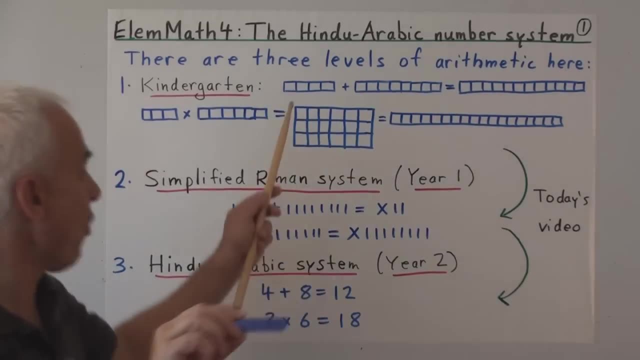 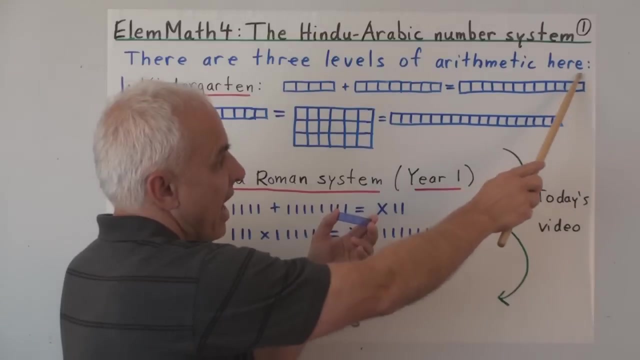 So I hope you can see that's a little rectangle with four little blue squares together. This could be a good model for the number four which is appearing right here. And a young person can say: let's say, we're trying to count how many letters the word here has. 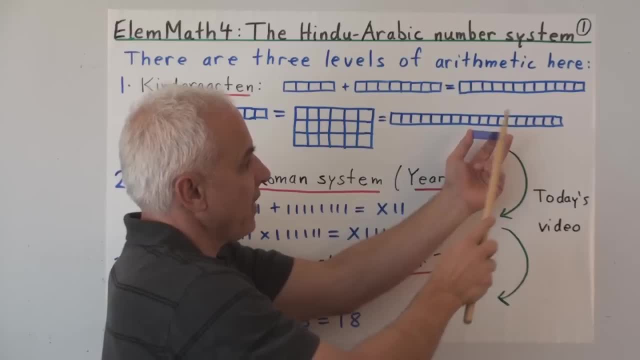 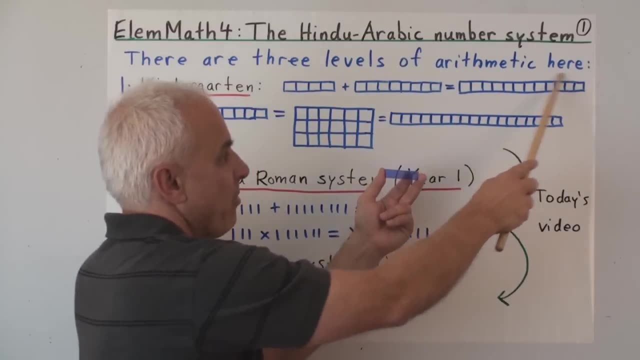 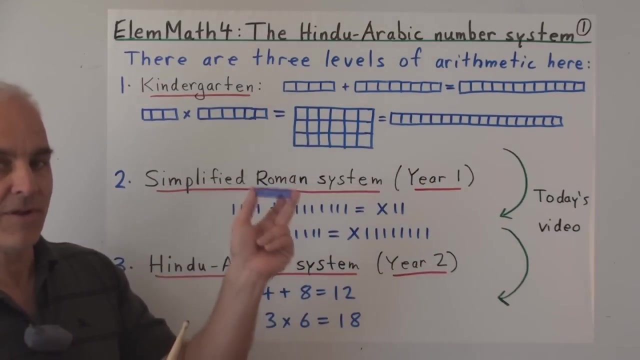 The person could count that by saying: well, there's the H for that That first one, E for that one, R for that one, E for that one. So the squares here exactly match up with the letters there. So we're counting the number of letters there and we're obtaining as a result this number. 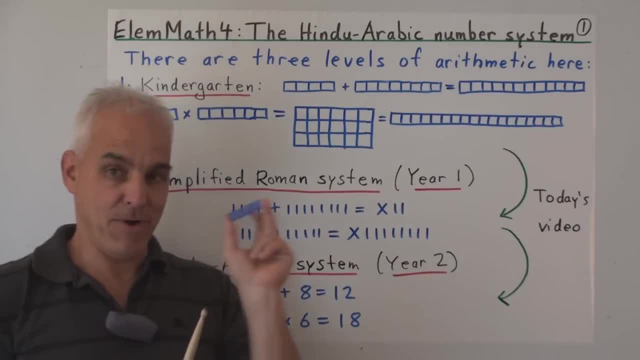 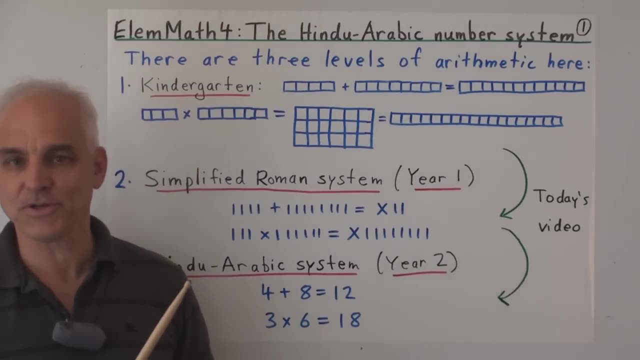 This is a number. That's a better way of thinking about what a number is actually than a symbol like this. Might appear a bit of a controversial statement, But I'd like you to think about this, This thing here, as being a symbol that represents this number. 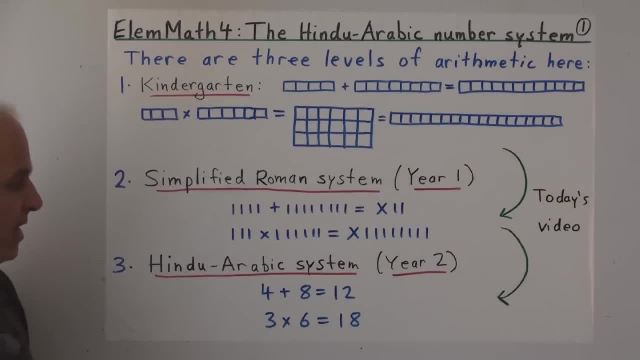 Or this number. So, in my view, to understand this Arabic system, one should really proceed in two steps, From the primitive system to an intermediate system, which I like to use, the simplified Roman numeral system, And then a second step from there to the Hindu-Arabic system. 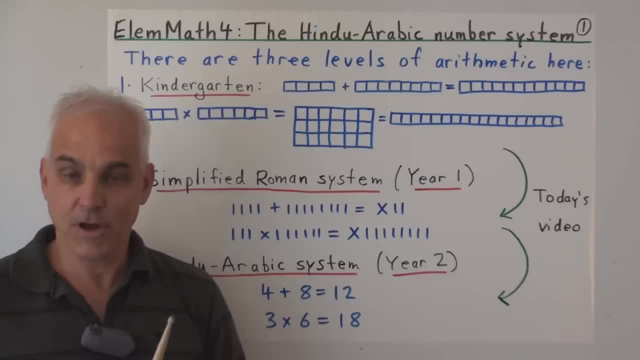 Makes the Makes things, in my view, a lot clearer. So that's the approach that we're going to take in today's video. We're going to talk about going from here to here, Introduce this simplified Roman system, And then we're going to talk about how to go from the simplified Roman system to the Hindu-Arabic system. 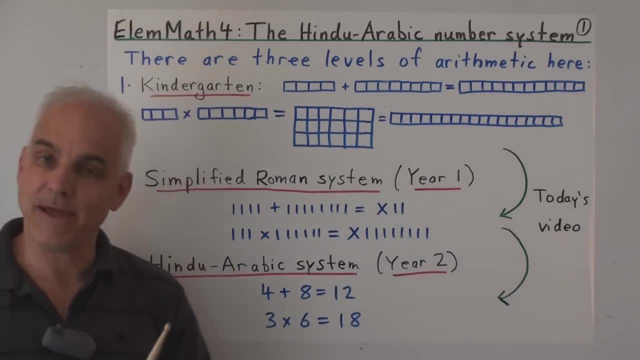 And one piece of technology that's going to play an interesting role is the abacus. The abacus helps us going from here to here. Okay, so a very important video. today We're going to introduce the Hindu-Arabic number system. 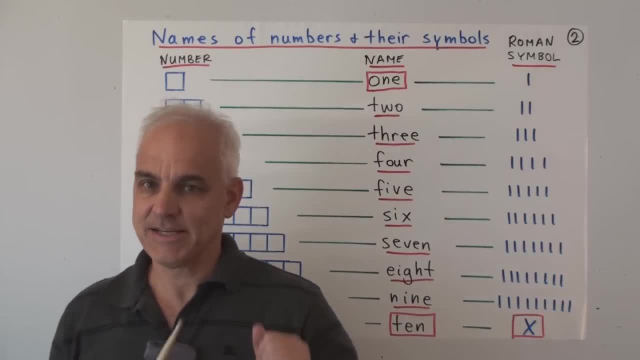 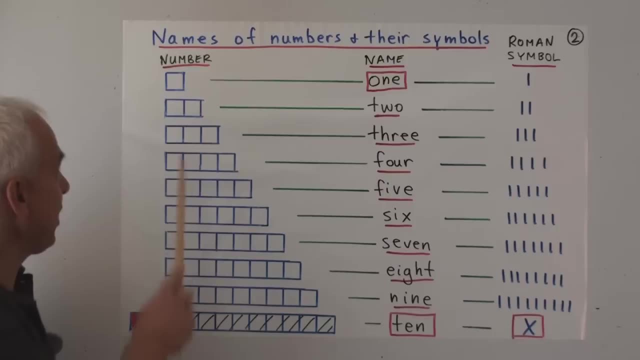 So a very good place to start is with the first ten numbers. They play a particularly important role in this number system. So here are the first ten numbers, written in our naive kindergarten approach, With rectangles divided up into a certain number of cells. So there's the number. 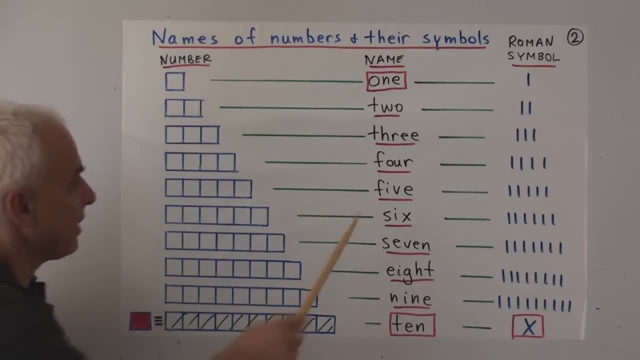 We were used to. So here are the various numbers, And here now we're going to introduce names for the numbers. Up till now we've only had the name for this one. We called it one, And all the other names were created from just repeating ones. 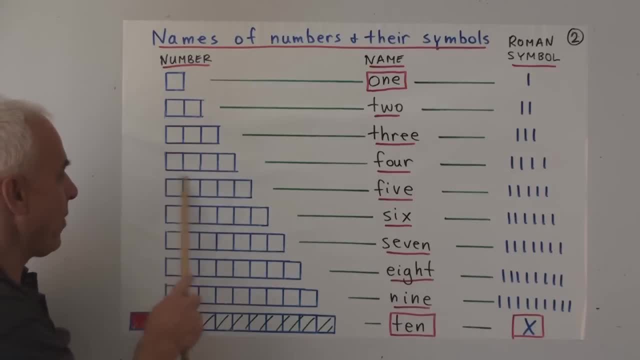 So we used to call this one, one, one, one. Now we're going to call this number four. Now I remind you that young people can talk long before they can write, So they can learn That this thing here is the number four. 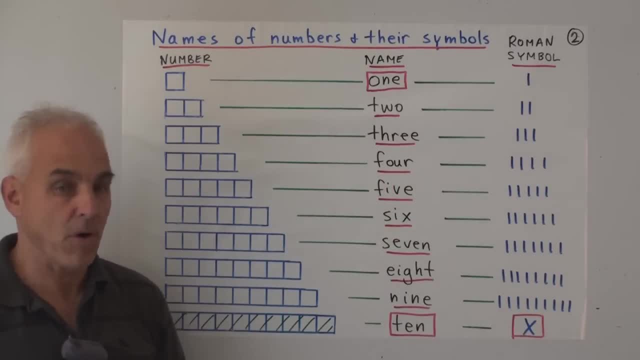 They can learn that word long before they learn how to read four, Or long before they actually learn our symbol for four. So that's the important thing To understand first. this is the number one, That's two, That's three, That's four. 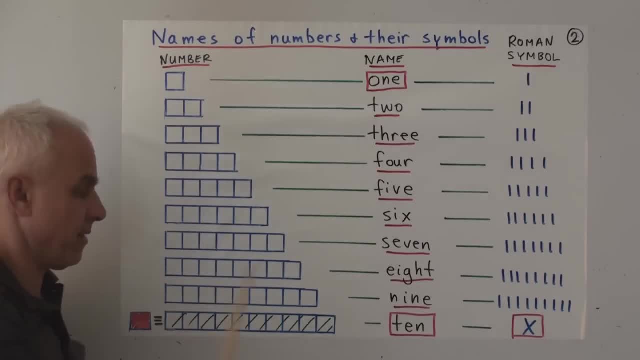 That's five, That's six, That's seven, That's eight, That's nine And that's ten. Now, every ancient culture that had a numerical system would essentially have done something like that. I think it's reasonably fair. It would have introduced names for the various numbers. 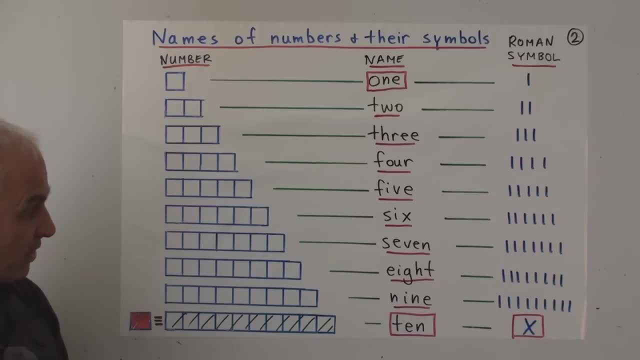 At least the first few. They may not all have introduced symbols for them, So later we're going to introduce the Hindu-Arabic symbols, which are yet something different from the names. But before we do that, we're going to talk about the Roman symbols. 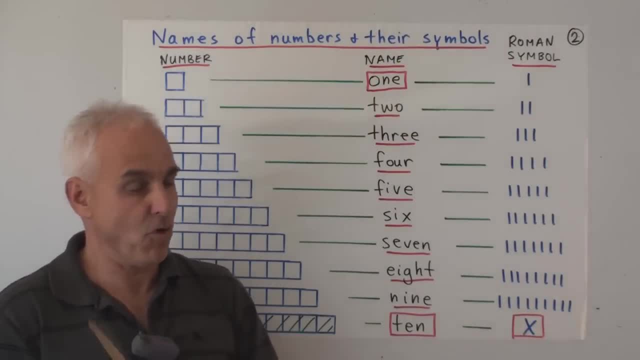 Or the simplified Roman symbols, Because this is a simplified Roman system here. So the simplified Roman symbols for these names. These numbers are just what you would expect. They're just strokes of ones, One being a single vertical stroke in this case. So the way we would write this number down on a piece of paper is just to make a single vertical stroke. 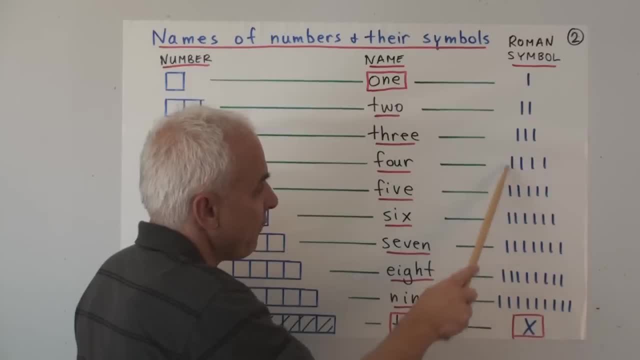 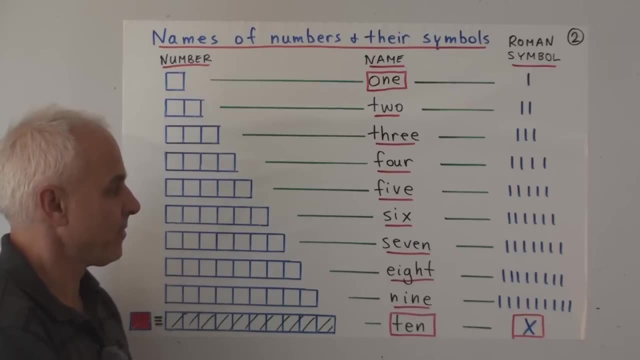 And now here's the number two, Three, Four, Five, Six, Seven, Eight, Nine And ten gets a special new symbol. Note that we're making a little bit of a departure from the last number. In the last video we said that it would be convenient to replace five with a V. 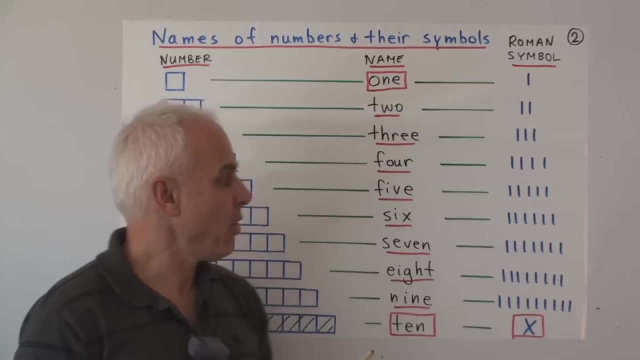 We're not going to do that this time. We're going to base things on base ten rather than on base five. That's an aspect of why this is called a simplified Roman system, So all the numbers have strings of ones associated with them up till ten. 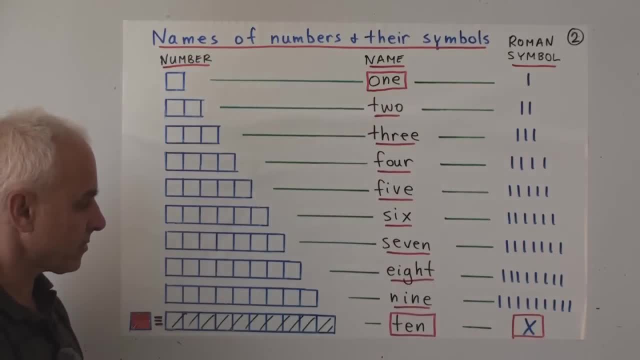 And ten gets replaced with this new symbol X. Now, on the pictorial side, we could also do something similar. Why don't we introduce a new kind of object that represents this big rectangle with ten cells in it? And we'll do that with color. 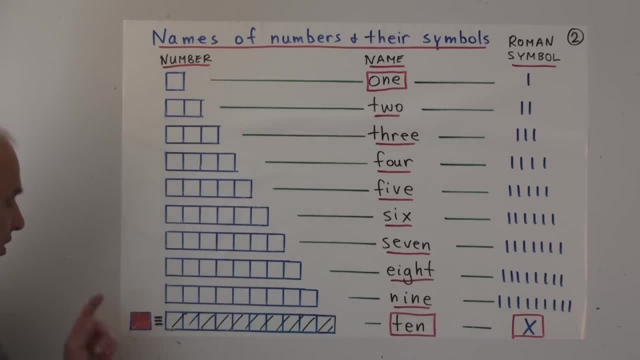 So we'll make a little square that's colored red And we'll agree that that one there is worth ten of the white ones. So that's our symbolic, or pictorial representation, Or pictorial representation of ten. So, for example, in blockus there would be a bunch of tens. 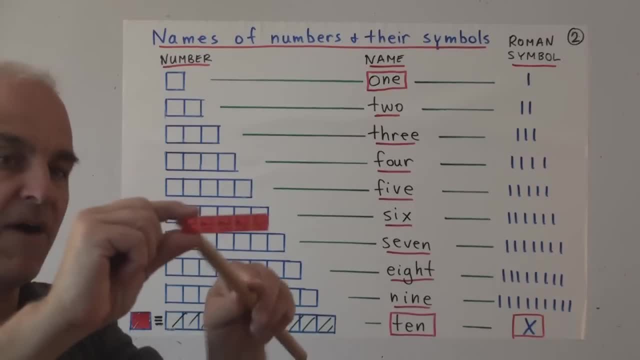 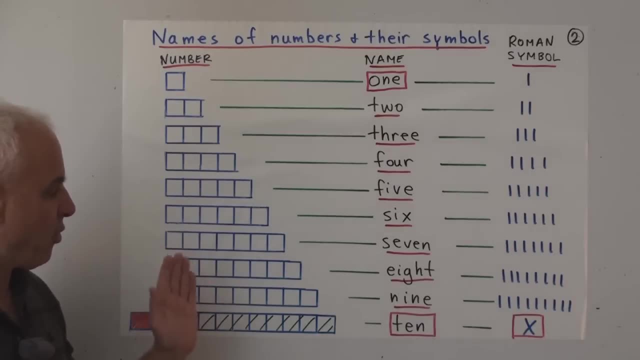 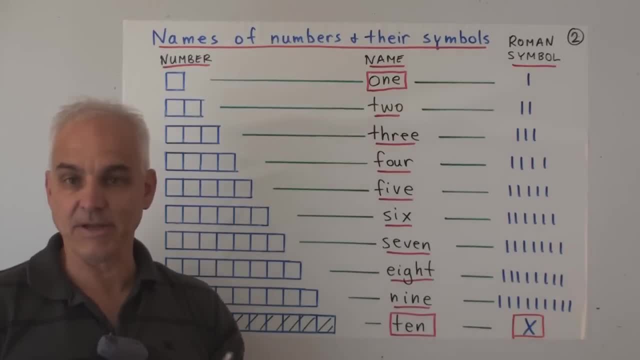 We've got the symbols for the numbers, If we're actually writing something down on a piece of paper. And at this level here, the crucial new thing- well, it's the idea that all the ancient civilizations had- is to introduce a larger unit to make it more efficient to write down larger numbers. 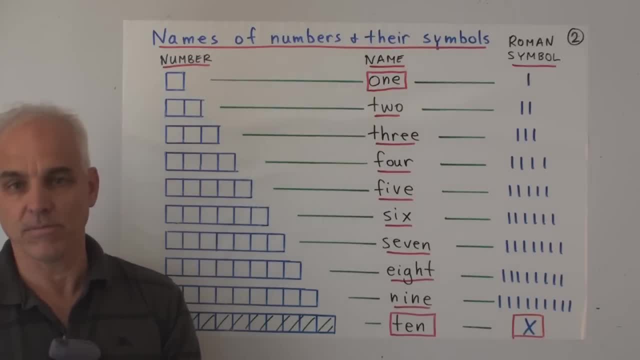 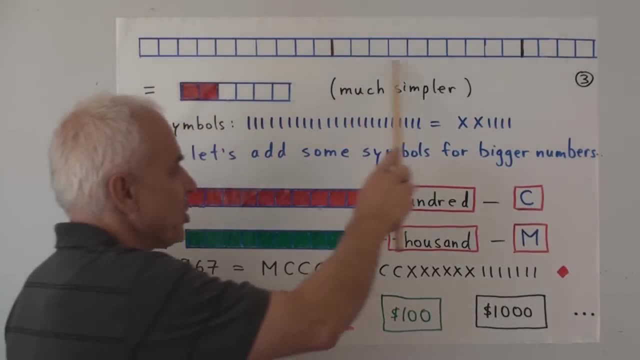 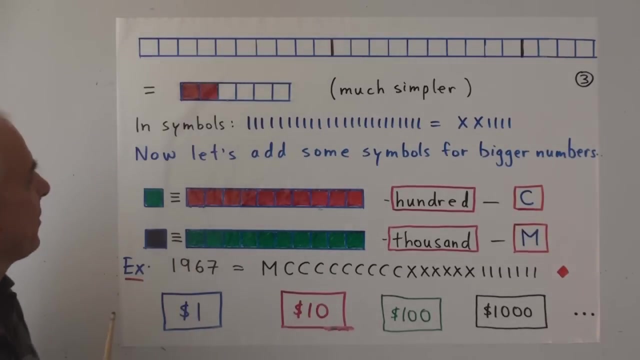 So that's our first new symbol, X representing ten. So how would this work in practice? Well, suppose we had a large-ish number- Say that one right there- And we wanted to write it in a more efficient, more compact way. 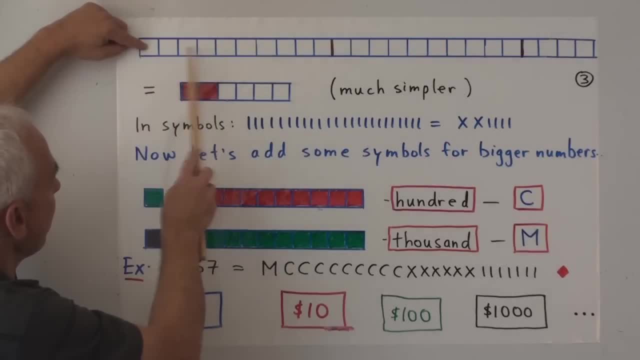 Then what we'd do is we'd look for a string of ten: One, two, three, four, five, six, seven, eight, nine, ten. So I'm using the fact that I've got names now for those numbers so I can count myself down to ten. 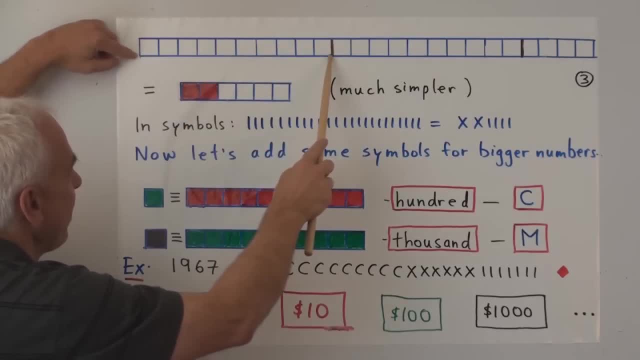 That's a string of ten. I can replace that whole string there with a single red one. A single red one is one. It's worth the same as these ten white ones or blue ones, And while there's some more room over here. 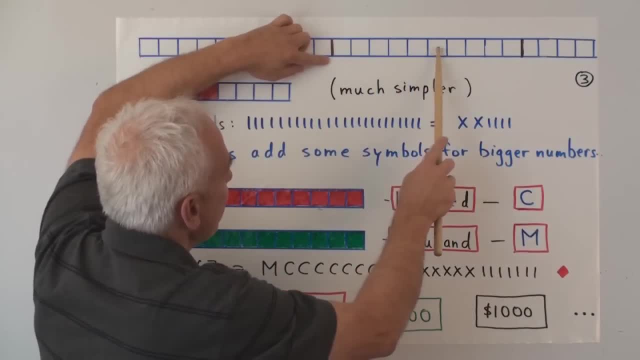 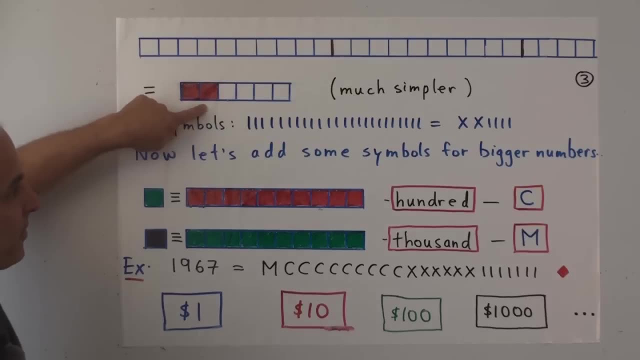 there's another ten right there: One, two, three, four, five, six, seven, eight, nine, ten, So that string there can be replaced by that second red one there, And there's four left over. We'll just copy them there. 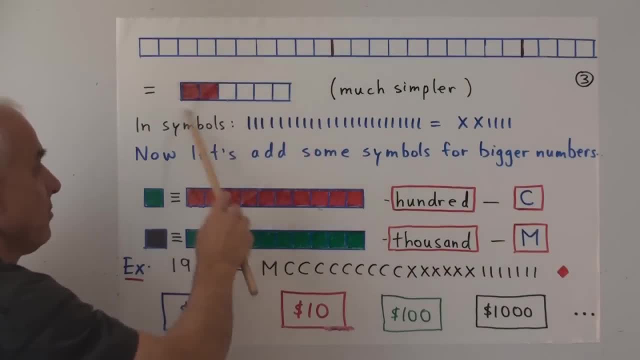 So this original number is now represented in this rather simpler form, a multicolored form, In a pleasant way. Now, in terms of our Roman symbols, the original number could be represented by all these ones, exactly 24 of them, in fact. 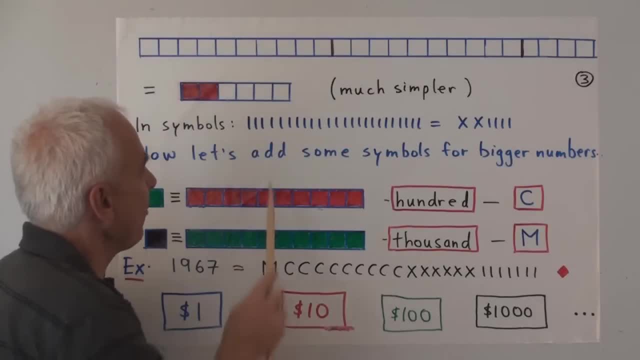 And we could have done the same thing on the level of these symbols. We could have counted off ten and replaced it with an x, counted off another ten, replaced it with an x, and then there would have been four left over. So this is the basic idea that underpins all the number systems in the ancient world. 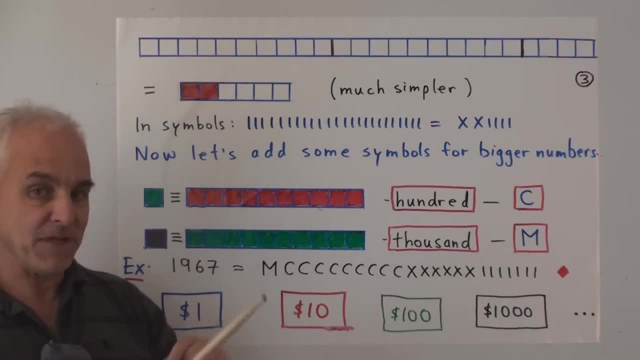 And we want to keep doing it. We want to keep introducing a few more bigger symbols to deal with ever bigger numbers. So the next one in our system is the symbol for a hundred or c, And that's going to be ten tens. 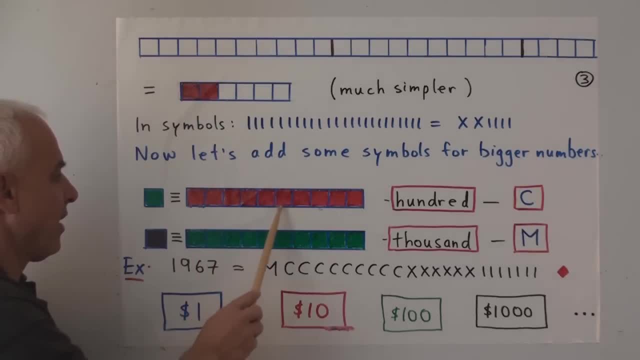 This is one ten, And here are ten of them, And we're going to agree that this string of ten tens can be replaced with one green square. We're going to call that green square a hundred and its Roman symbol will be c. 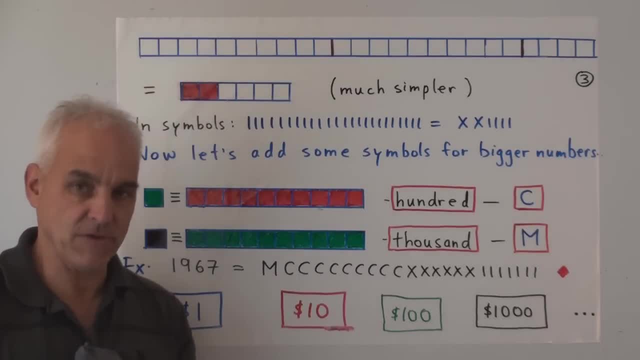 So that's the same as the symbol that the actual Romans used for a hundred c for century, And then one step further, ten hundreds, all in a row, can be replaced with one black square, which we'll call a thousand, and its symbol is m. 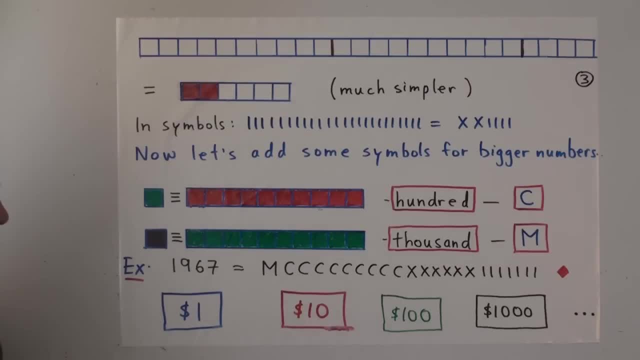 like for millennium. So for example, nineteen, sixty-seven, or the number one thousand nine hundred sixty-seven in our Hindu-Arabic notation would be written as one thousand, taking care of that. and then we need nine hundred, so a hundred is c. 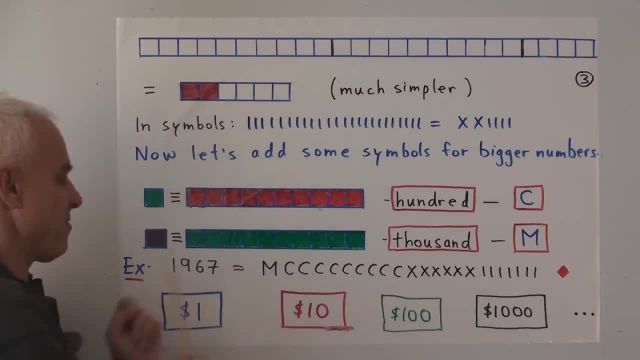 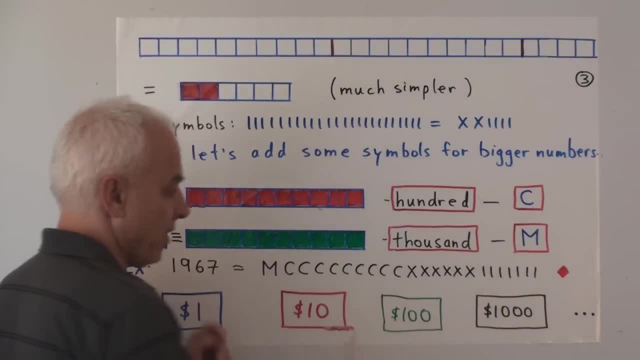 and seven ones left over there. they are there, And a very nice way of thinking about what's going on here is that we are introducing higher denominations, just as we do with money. So instead of having lots of one dollar bills, 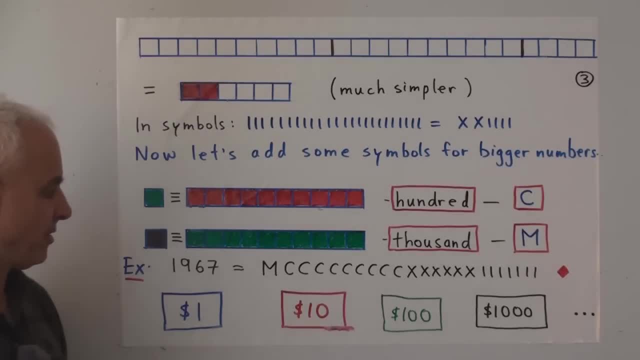 or one dollar coins. we introduce a ten dollar bill- maybe it's red corresponding to this, and then we also introduce a hundred dollar bill that's green and a thousand dollar bill that's black, and what we're saying here, for example, 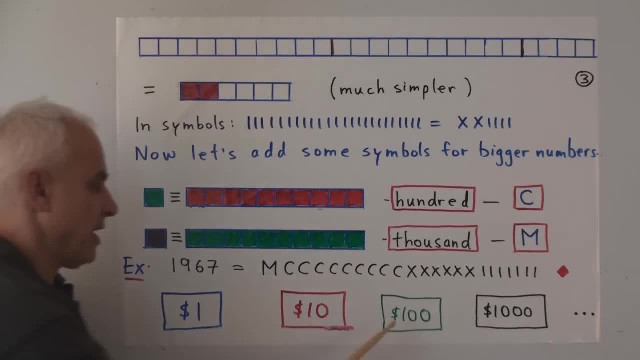 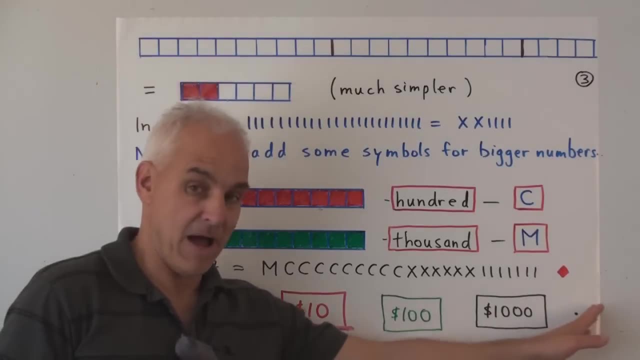 is that ten of these equals that, ten of these equals that. ten of these equals one of those. And we could conceivably introduce some higher denominations, but for now we'll just pause at the m. The Romans, in fact, didn't introduce anything bigger than m. 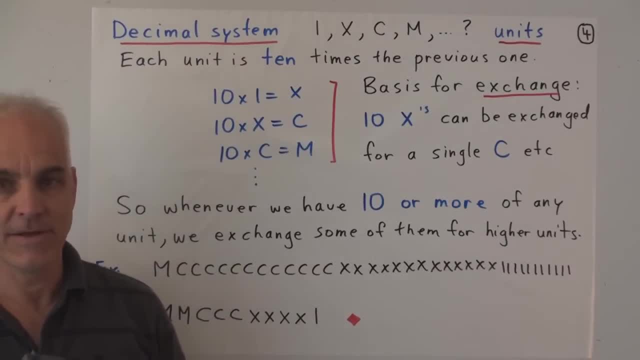 This is truly a decimal system, decimal being a word coming from the Greek for ten, because our various units, starting with one and then ten, and then a hundred, and then a thousand, they're all ten times the previous one. So ten times one is x. 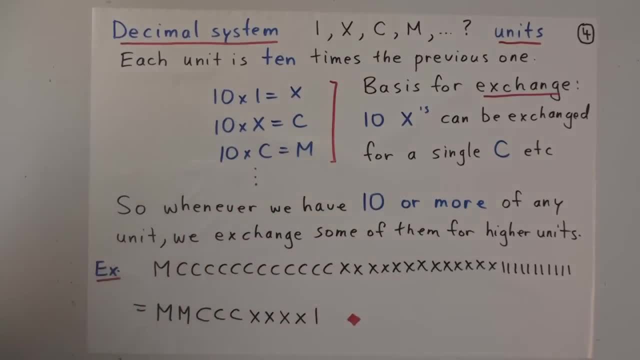 ten times x is c, ten times c is m, and so on. That's what we mean by a decimal system, And we can think about this, just to iterate it again, that this is a basis for exchange, that what we're saying is that 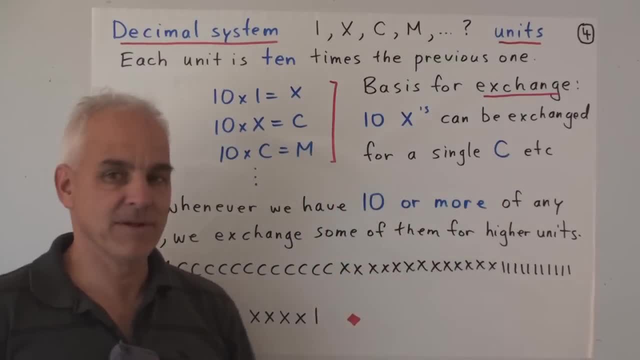 ten x's can be exchanged for a single c. It's like a bank. if you have one c, it's like one hundred dollar bill. you can trade it in for ten, ten dollar bills. So arithmetically, ten x's. 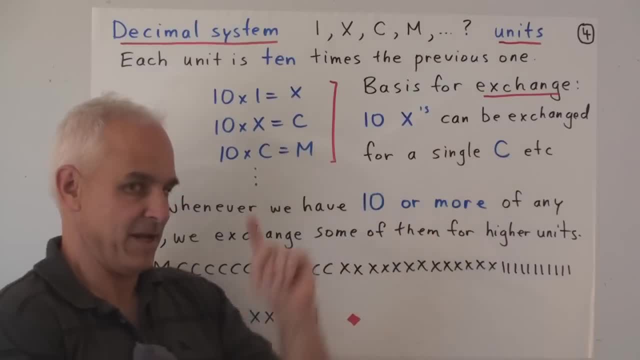 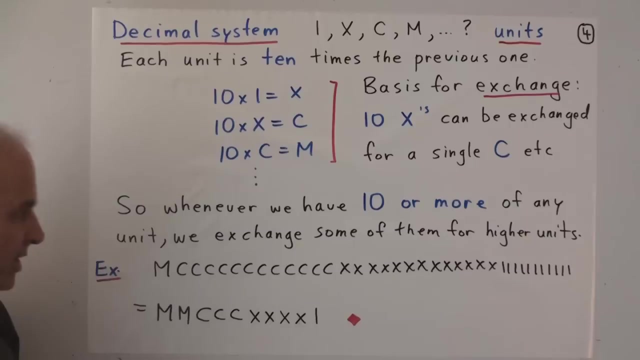 in other words, that many x's equals that many c's, And that many c's equals that many m's. So this has an obvious but kind of important consequence. The consequence is that whenever we have ten or more of any of these units, 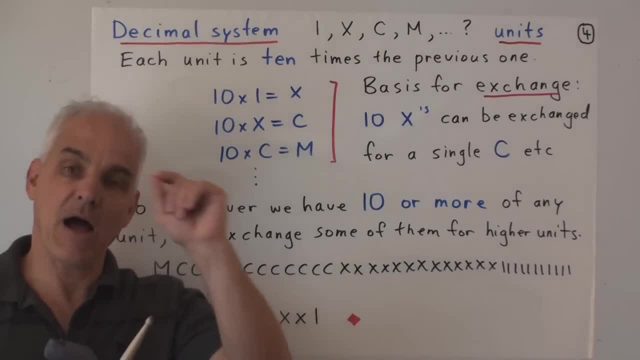 we can exchange some of them for higher units. Whenever we have ten or more, we can go to the bank and get a bigger unit in exchange for ten of the ones that we've got, making our number more compact. So, for example, 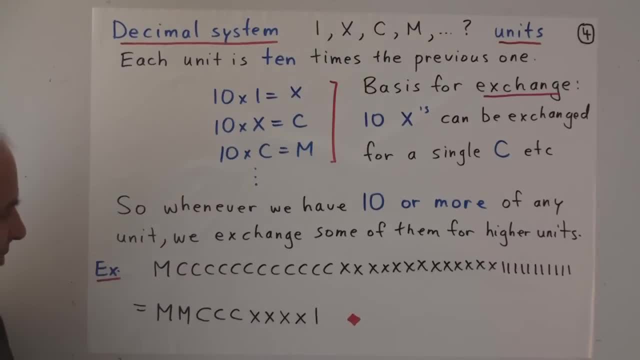 here is a number in our simplified Roman system. It's got one m, it's got a whole bunch of c's, a whole bunch of x's, a whole bunch of ones, And this is not the most efficient way of writing this. 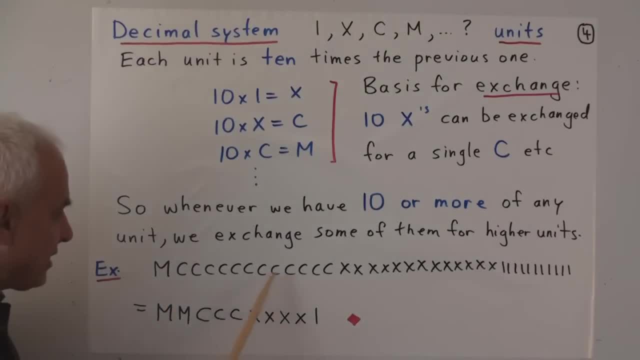 because there's, for example, ten c's here somewhere. Let's count them One, two, three, four, five, six, seven, eight, nine, ten, So those ten c's there can be replaced with a single m. 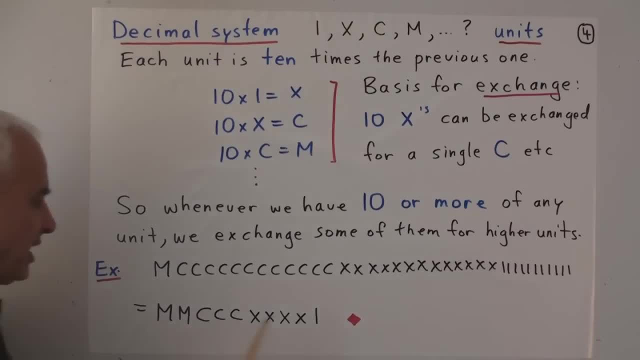 We might as well do that. That makes everything shorter. We still have two c's left over. Where did this third c come from? Well, it came from ten of these x's: One, two, three, four, five, six, seven, eight, nine, ten. 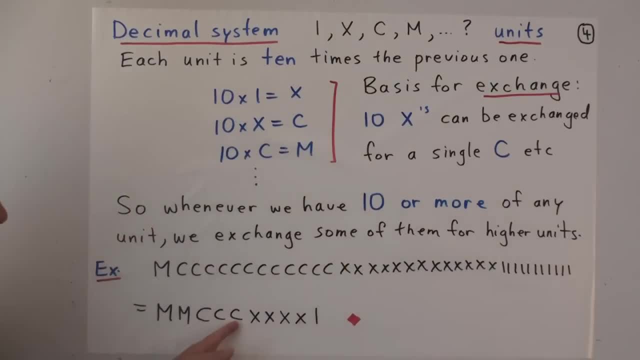 So those ten x's there can be traded in for one c, Leaving still three more x's, But that last x there, well, that's the result of trading in ten of these ones: One, two, three, four, five, six, seven, eight, nine, ten. 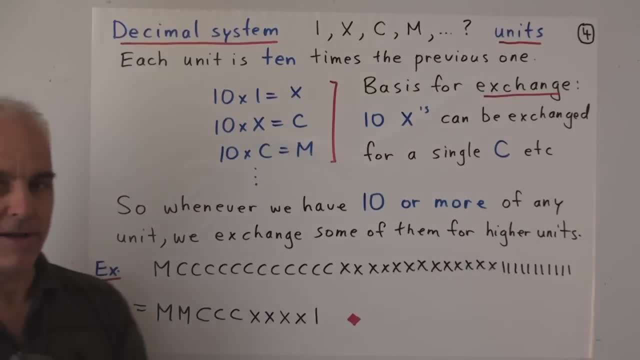 That's all of them except for one, So it'll still be a one one left. So in this way, if anybody writes down one of these Roman numbers, we can simplify it by looking to see whether there's ten or more of a unit. 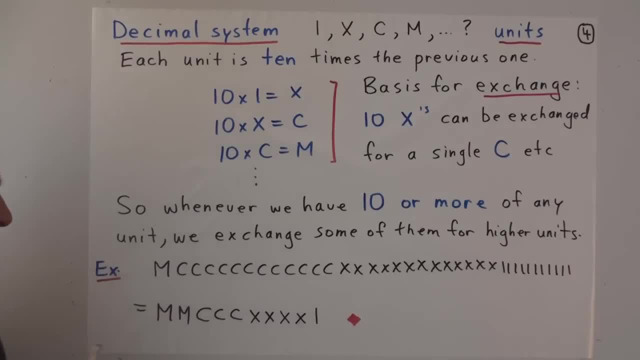 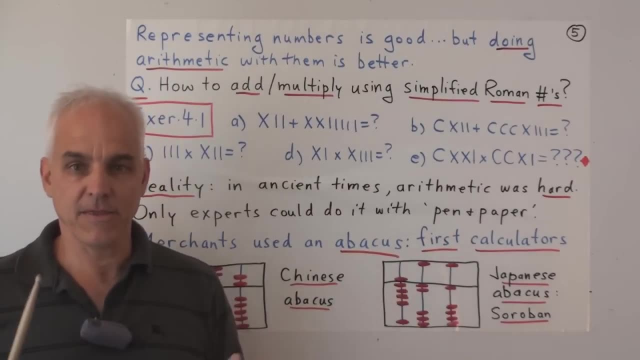 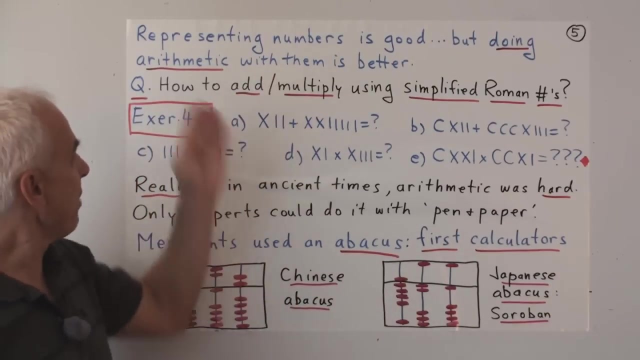 And if there is exchanging those ten for a higher unit. So I think you understand pretty well now how to represent a number in this simplified Roman system using ones x's, c's and m's. So that's good, but doing arithmetic with them is even better. 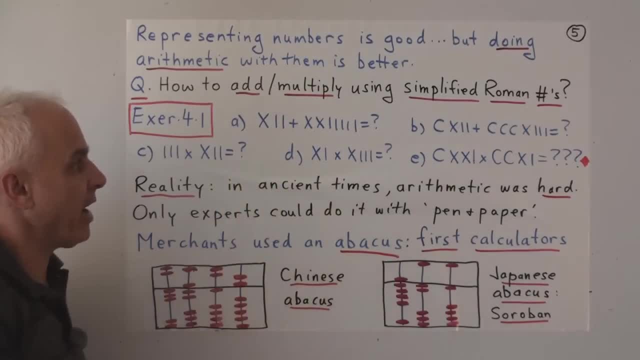 So a natural question is: how are we going to add or multiply using these simplified Roman numbers? So here's. the first exercise for today is to have a look at a few examples of arithmetic with these Roman numbers and see if you can figure out. 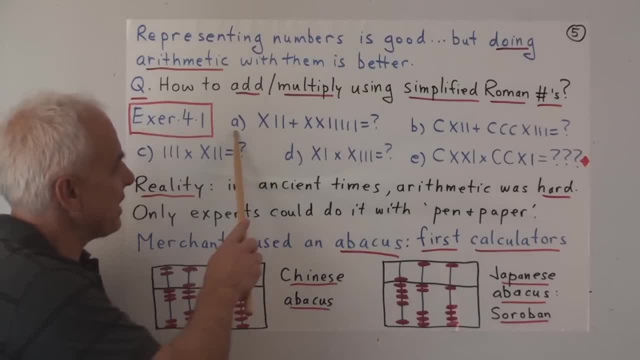 what the answer is. So this first one. for example, we had this Roman number which we would read as ten one one, and then plus ten: ten one, one, one, one one. Or we could say ten ten five. 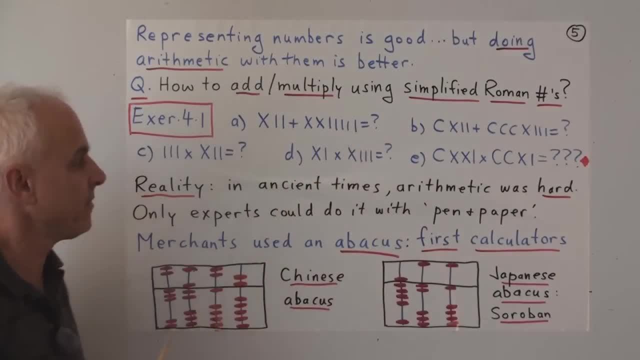 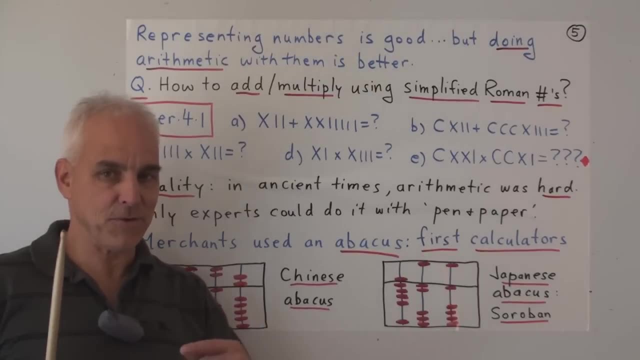 because we know one, one, one, one one is actually five. So what happens when we add these things? Well, I remind you, you're not allowed to convert to the modern Hindu-Arabic notation and then use whatever arithmetic skills. 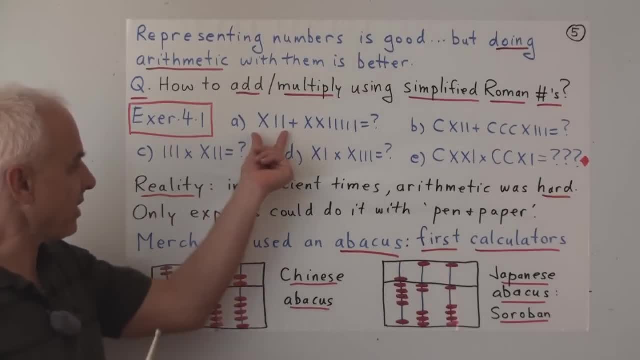 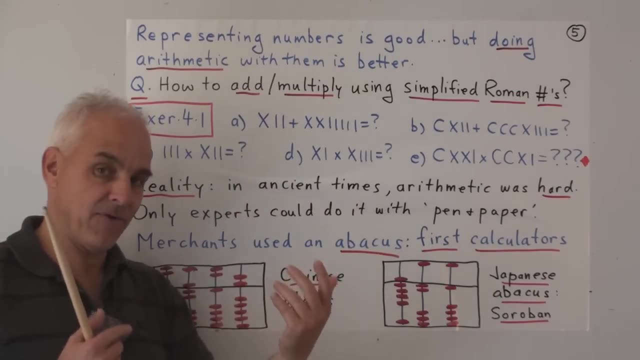 you've already learned. The idea is to recognize that these numbers represent ultimately long rectangles And we want to convert things into the rectangles and then sort of imagine what's happening at the level of rectangles and then convert back to something that's Roman. 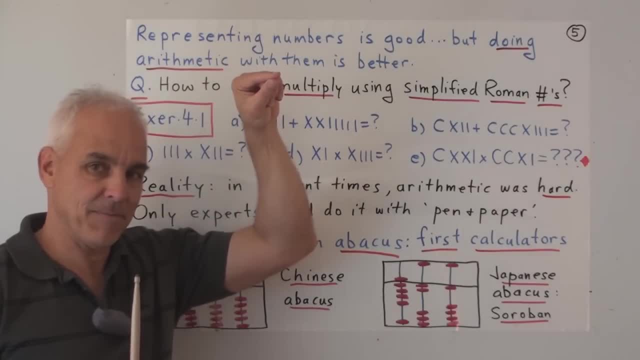 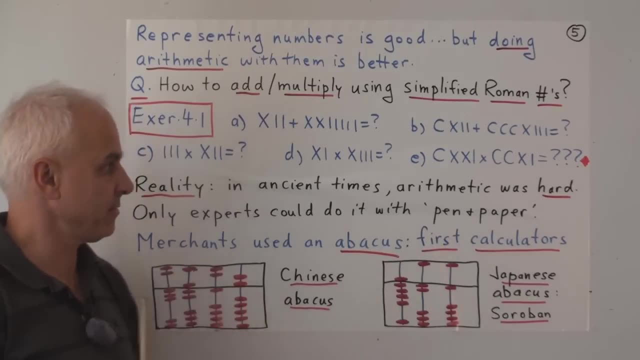 So I want you to go back to the more primitive system to understand what's happening, not to the more advanced system of the Hindu-Arabic numbers, which we haven't gotten to yet. Okay, it's of course a little bit more complicated. 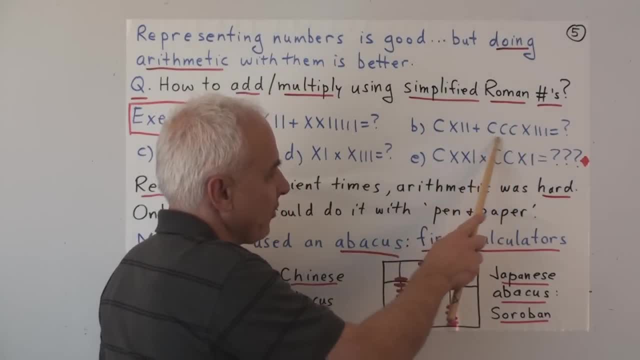 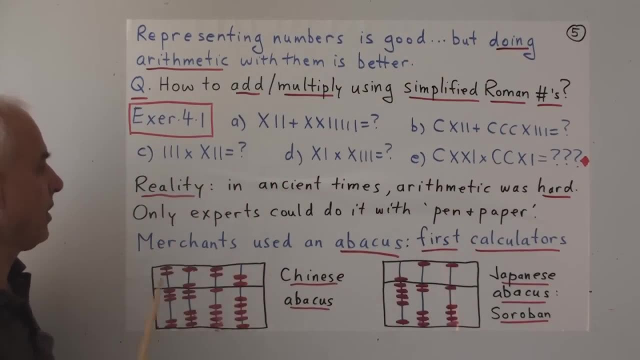 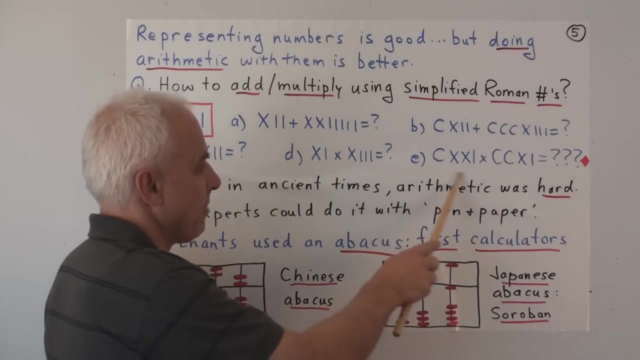 when the numbers get bigger. Here's some numbers with some hundreds in it. Here's a multiplication Three times ten two. Here's ten one times ten three And here's some product involving some hundreds. This is going to be very challenging for you. 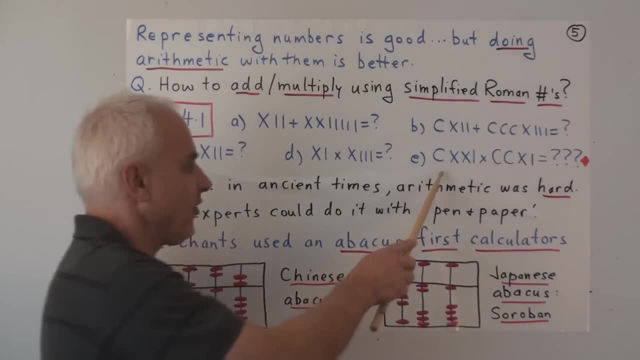 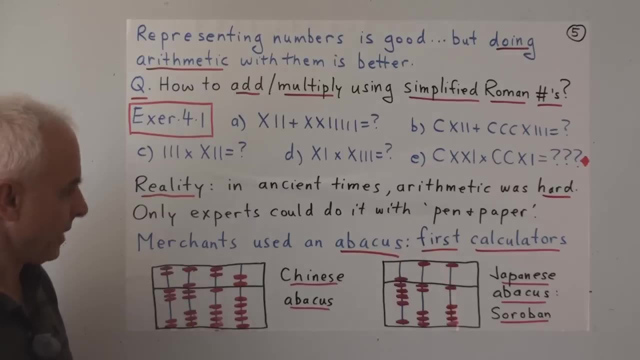 This ought to be very challenging for you. alright, It ought to be. If this is easy, then well, either you're very gifted or maybe you're cheating a little bit. See, the reality is that in ancient times, arithmetic was hard. 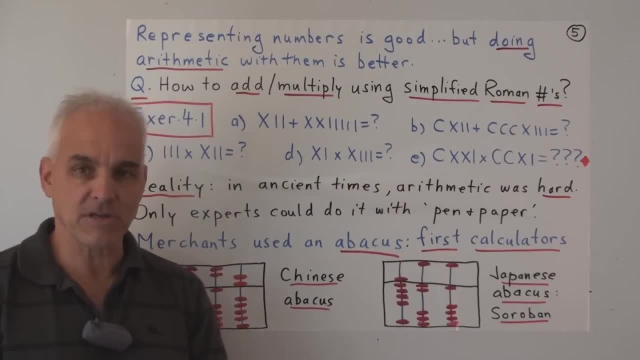 Questions like this would have stumped most people. They wouldn't have known how to do these questions just by hand. Only experts could do it with a pen and paper. First of all, pen and paper. well, paper would probably have been relatively expensive. 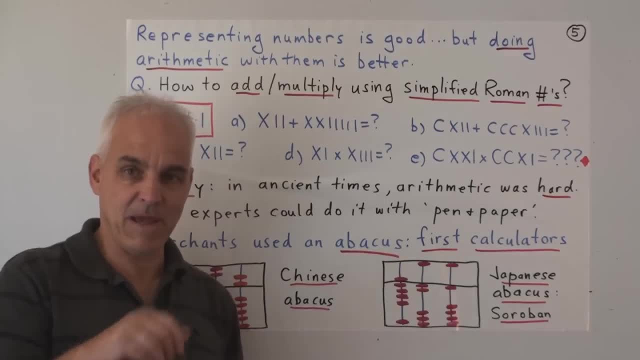 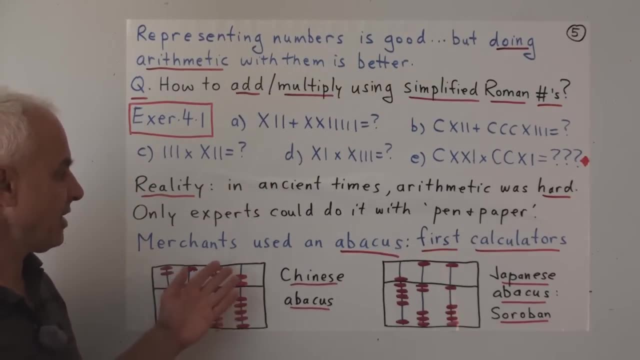 and people probably wouldn't have been happy to waste paper making long arithmetical calculations, So what they actually did instead was to use calculators Well an abacus. So this, of course, probably arose most often in merchants making commercial transactions. 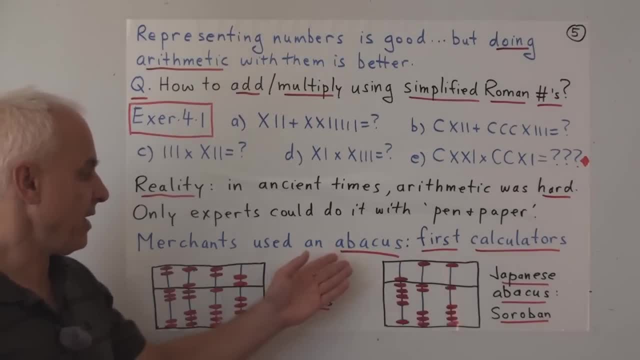 where abacus, where you need to make calculations, and the abacus, or accounting frame, was a very important technology that was almost universal across many, many cultures. So here's an example of a Chinese abacus, sort of a simplified one, not as many columns, as usual. 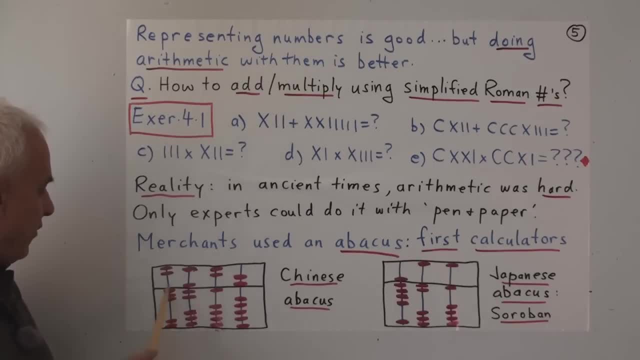 So there's sort of a bar somewhere, and then there's sort of five beads on each rod below the bar and two beads above it. There's also a Japanese abacus called a soroban, which is a lot like this, except that there's only one above the line. 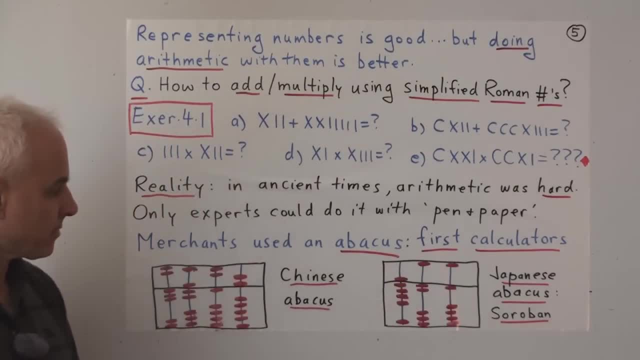 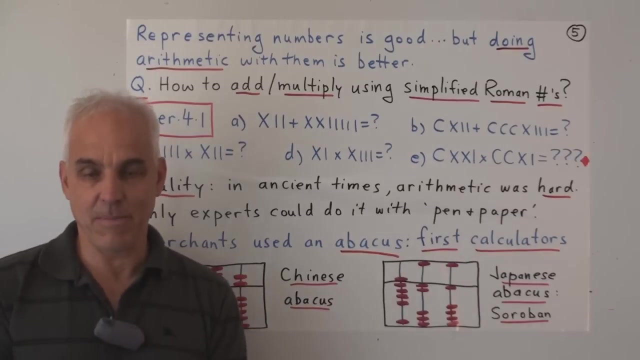 Five below the line and one above the line. I told you I'm not very big on technology, but in fact this is quite a good technology to help us learn to do arithmetic. Let's have a look at an even simpler kind of abacus. 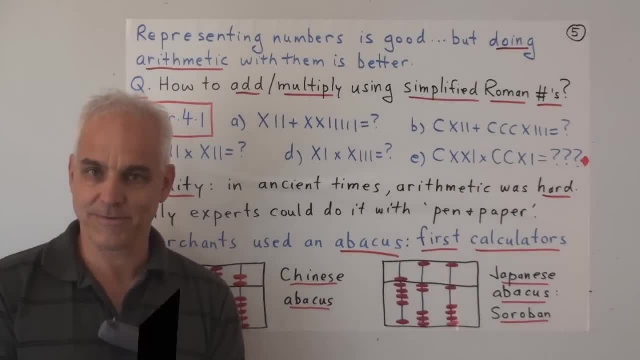 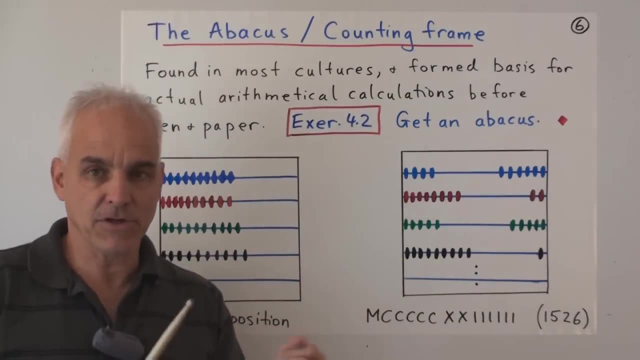 that preschool kids often play around with. So an abacus is a device, a physical device to represent numbers and to allow you to do arithmetical operations like addition, subtraction, multiplication, perhaps even division, And most cultures had some kind of mechanical devices. 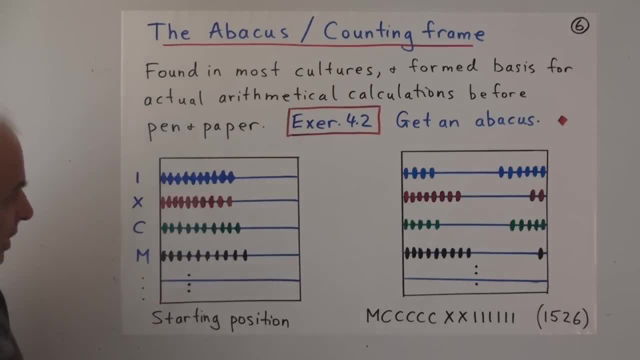 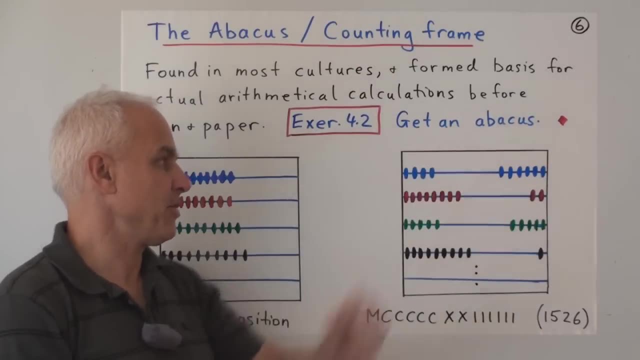 that were in this direction. So exercise 4.2, why don't you go and get yourself an abacus if you don't already have one? They're a very good tool for learning arithmetic and becoming familiar with the way arithmetic works. I'd be very happy if young people in years K-6 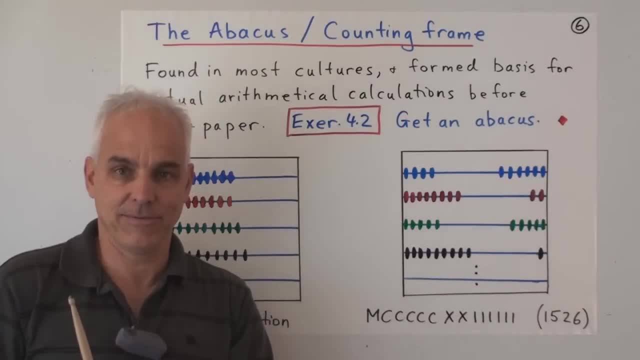 were able to trade in their calculators for abacuses. That'd be a great way of doing it. It's a great way of improving immediately mathematics education across the world. This, I think, is appreciated in Asian countries, but in Western countries it's still not very well accepted. 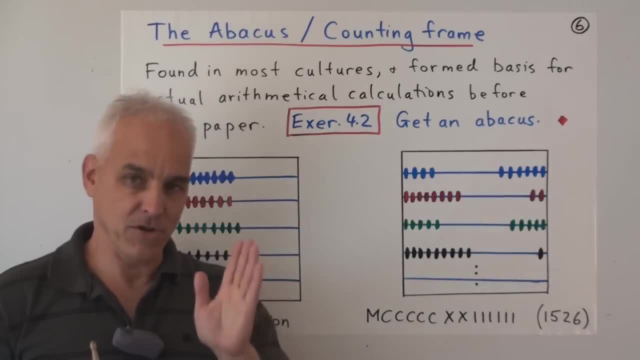 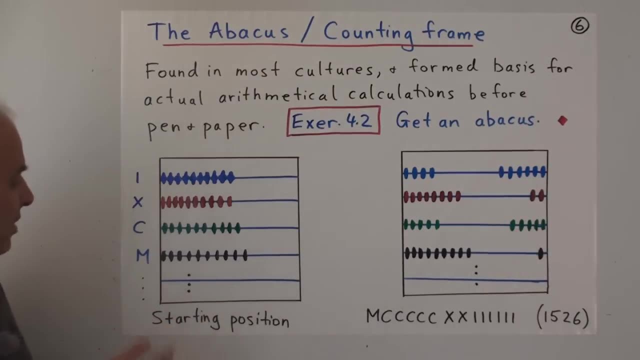 But an abacus is far superior to a calculator when you're trying to learn arithmetic and mathematics, believe me. Okay. so here's a very simple kind of abacus that very young children can use. We have a frame with some rods, and on these rods are little colored beads that can slide. 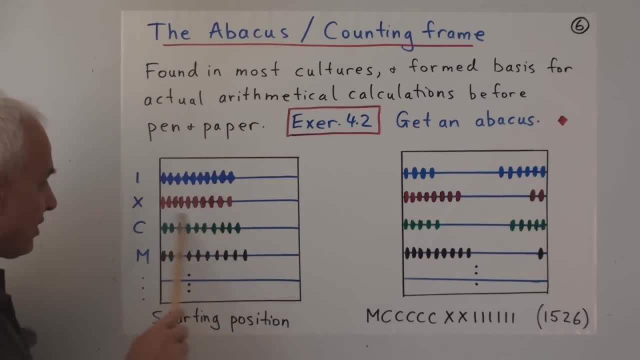 And there's typically ten of them. So we've got ten blue ones, ten red ones, ten green ones, ten black ones, And I've used these colors because they represent the colors that we've been talking about, representing ones, tens, hundreds and thousands. 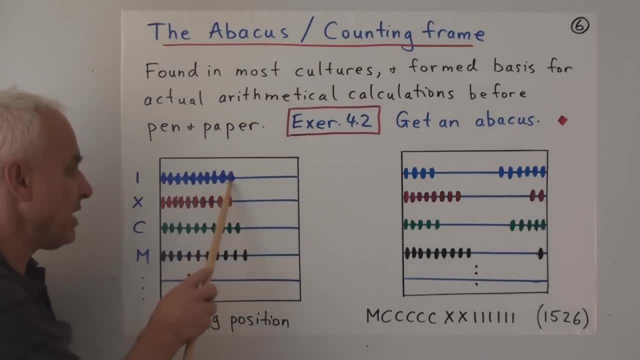 So what we're going to do here is we're going to think about each one of these beads as representing one, And each one of these red beads as representing a ten. So a red bead is just like a little red square, And a green bead is representing a hundred. 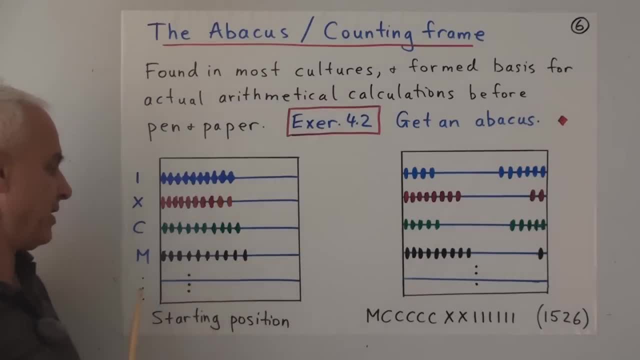 That's just like a little green square And a black bead is representing a thousand, like a little black square, And if we wanted to, we could have more rows and we could think about bigger numbers, bigger units as well, But we'll stick to these four colors for now. 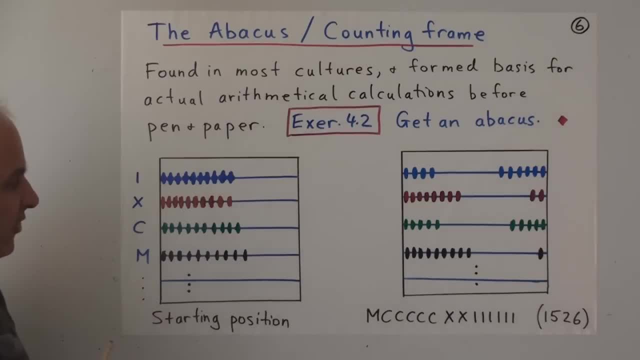 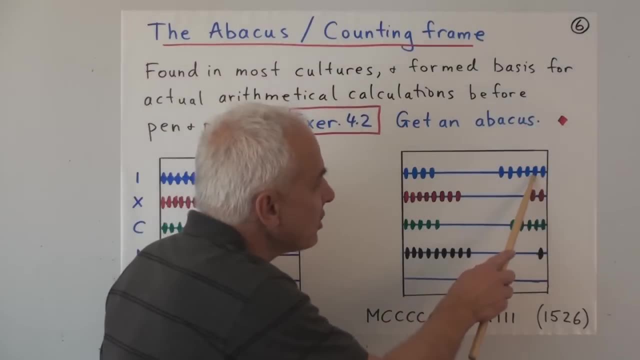 So how do we represent a number in this system? Well, we slide over. We've got a certain number of beads. So here we've slid over one, two, three, four, five, six of the blue ones. The blue ones represent one. 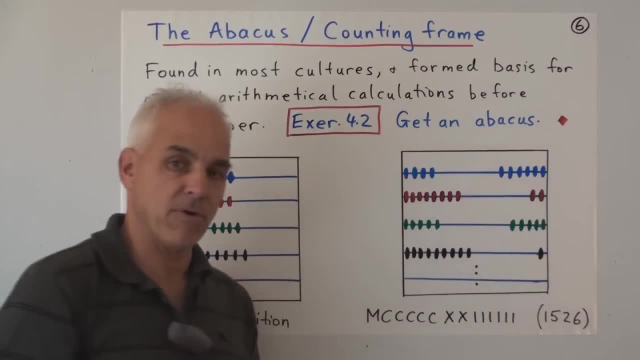 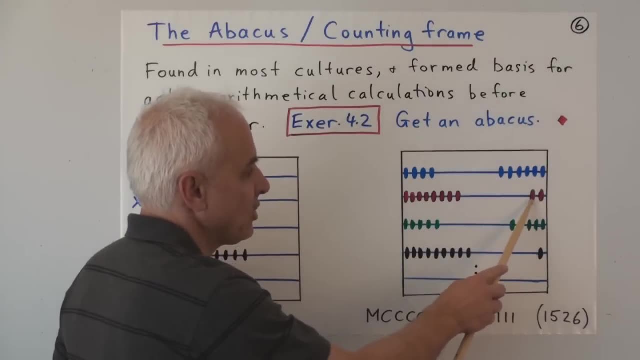 So we've really slid over six. So this by itself represents the number six. And we've also slid over two of the red ones, So each one of those is a ten. We've slid over five of the green ones. There they are there. 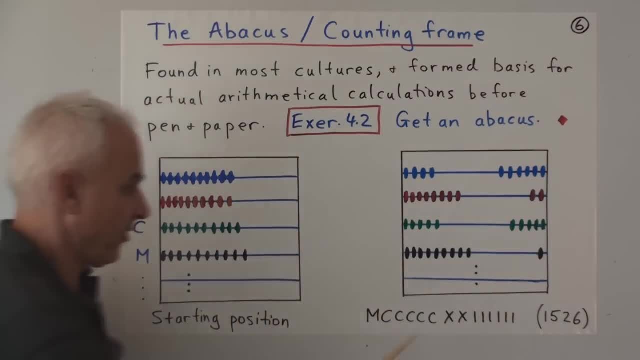 Each one of those is a hundred. We've slid over one of the black ones. There it is there. So what's appearing here on the right-hand side represents a certain number, And we can write down the Roman symbol for it very easily by starting from the bottom here with this thousand. 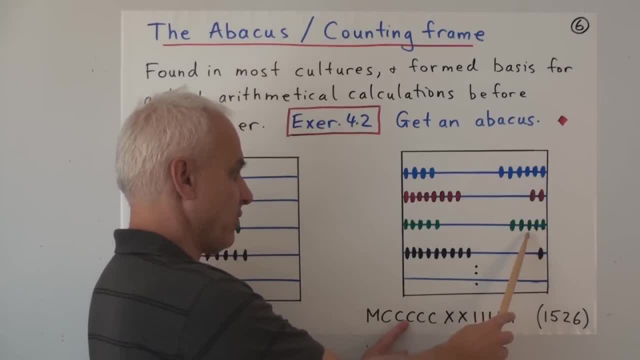 writing an M. Then for each of these green ones we'll write a C, because they all represent a hundred. So we get C, C, C, C, C, And then we have a couple of X's representing the tens, And then we have a couple of ones. 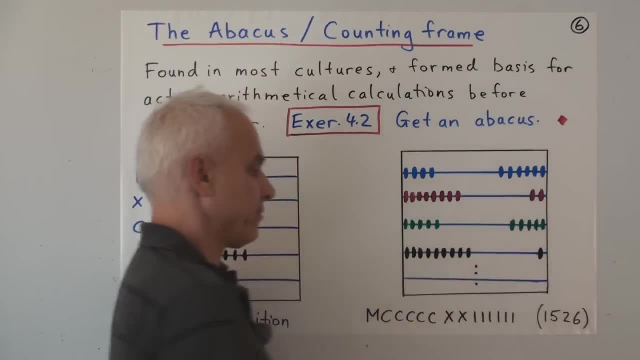 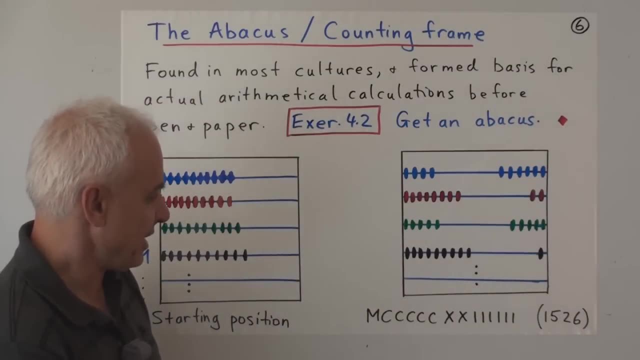 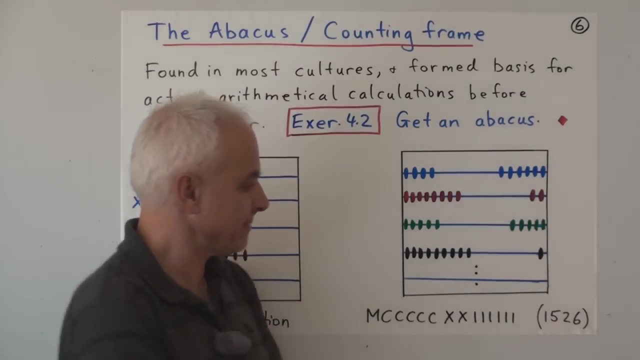 representing these unit ones up here in blue. So going forward a few hundred, maybe a thousand years, here is the Hindu-Arabic numeral for this. We would call this 1526.. So how are we going from this or this to something like this? 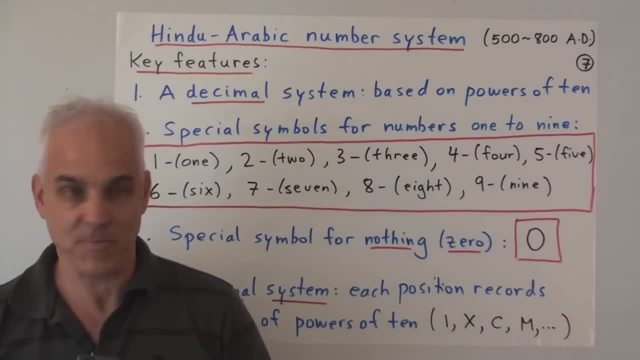 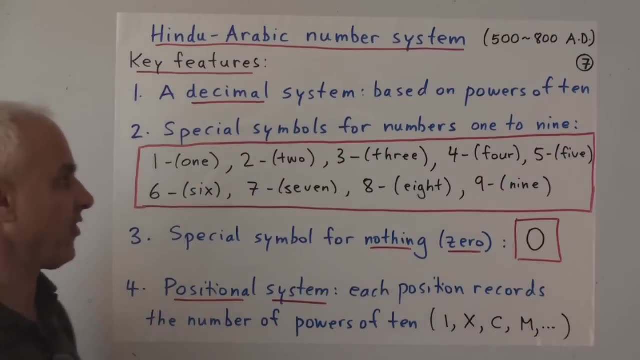 Well, it's time to introduce our Hindu-Arabic number system, which has a number of key features. The first is that it's a decimal system. It's based on powers of ten. The second is that there are special symbols now for the numbers one to nine. 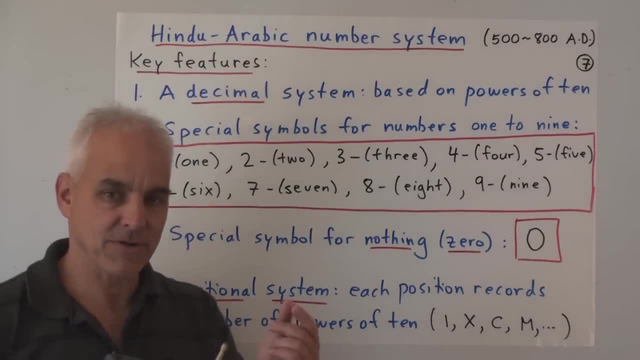 We introduce more compact symbols, sort of separate symbols for each of the digits. We don't just write one and then one-one, and then one-one-one for one, two, three. We now introduce these symbols: one, two, three, four, five, six, seven, eight, nine. 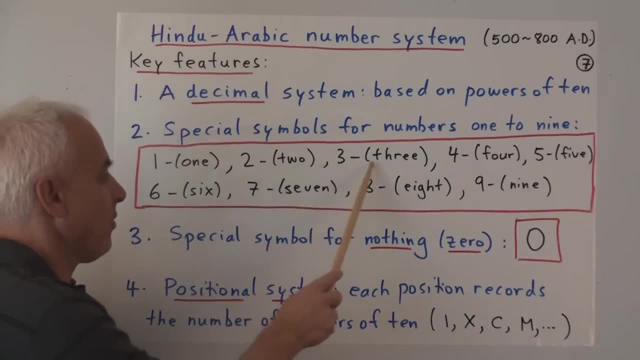 for the respective numbers whose names are one, two, three and so on. Of course, these are very familiar things, but they've evolved over time quite a lot, Although the Hindu-Arabic number system was developed somewhere around 500 to 800 AD. 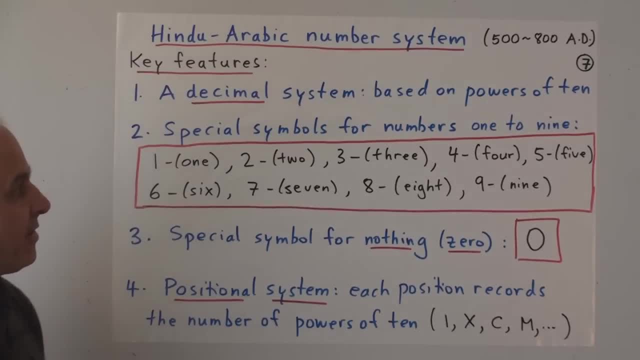 we don't actually know who exactly was responsible. It was probably a number of people making contributions over a long period of time. These symbols or these digits actually evolved over the years, were modified by the Arabs later on and they probably achieved this kind of form. 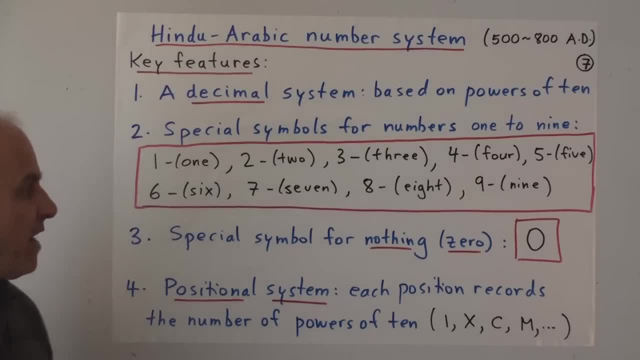 only in the relatively recent past, maybe the last 500 years or so- And in fact there's still modifications going on to these digits even today. So many of you younger people perhaps will not write a seven the way I do, So I was taught to write a seven. 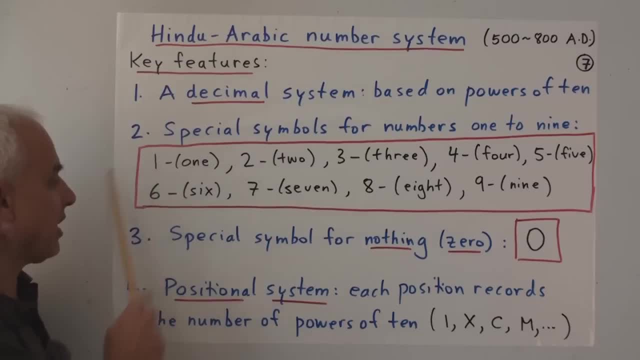 with a little bar across it to not get it confused with a one, Because back in my time one often wrote a one with sort of a base on it and then a little flag flying there, And then it became a little bit easy to confuse the one and the seven. 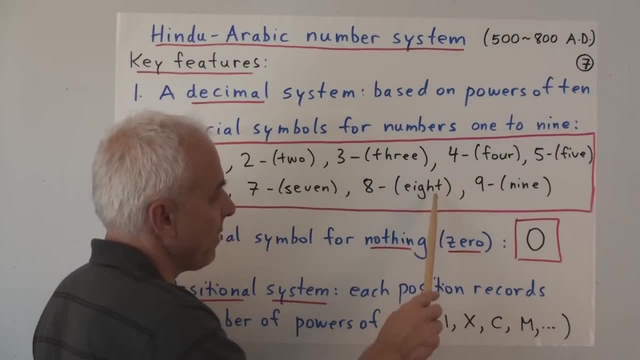 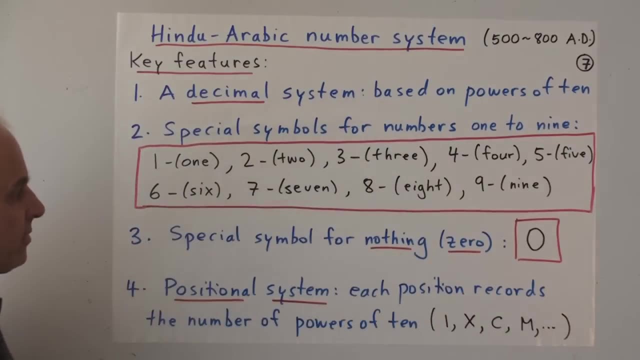 Another point is that the four that I've written here is somehow different from other fours Sometimes. this one here is sort of diagonally, so that a four looks more like this. You'll all recognize that too, And I just note, even with my daughter. 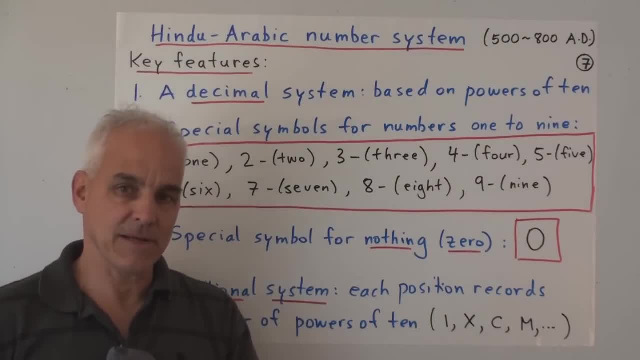 the way she learns to write these numbers in school is different from the way we were taught to write them, So there's still an evolution going on. Maybe in a hundred years from now they'll look a little bit different yet again, But anyway, 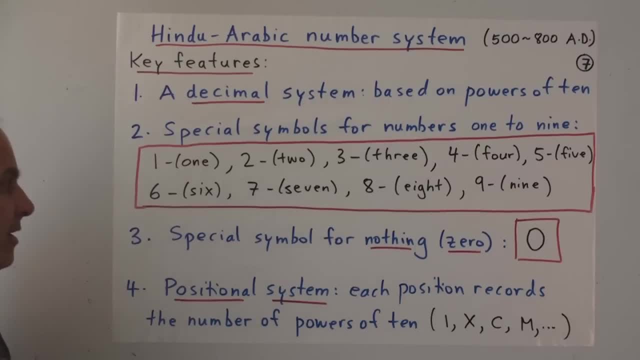 this was one of the very important developments, contributions that made the system work, that we have separate symbols for the numbers from one to nine. And then the third key feature, which is probably the most important one, even though it looks like the most inconsequential. 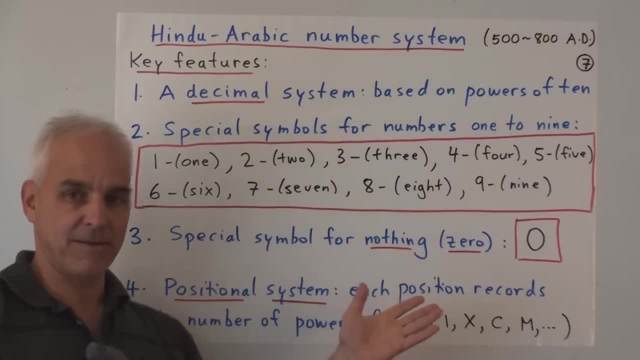 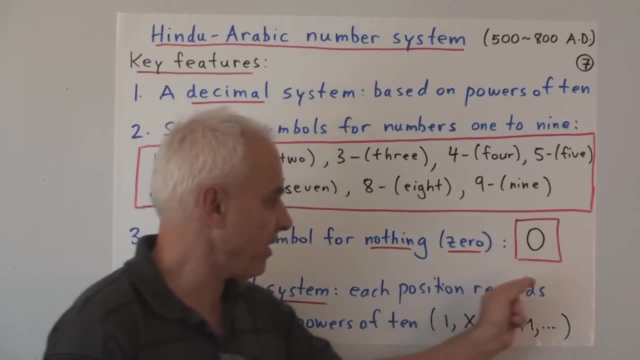 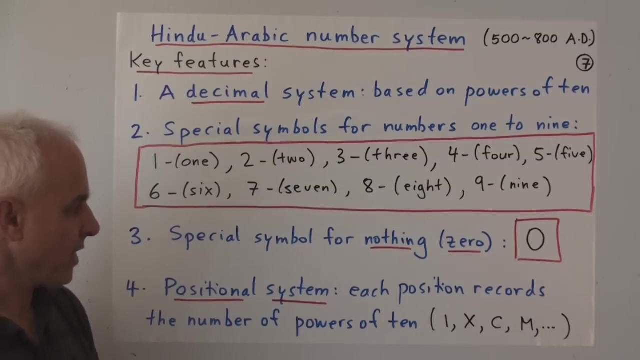 is that we have a special symbol for nothing. We call nothing zero. That's the number zero, And we actually represent it with, in this case, a sort of a circle or elongated circle. It's important that nothing has a symbol associated to it. 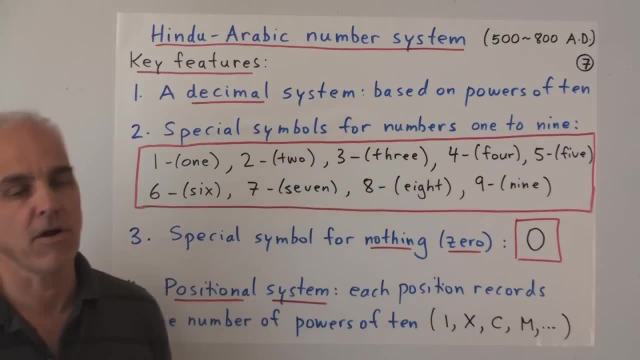 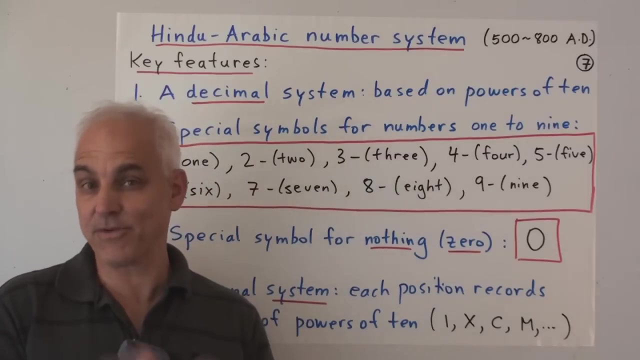 We saw that actually even when we were counting in one of our first videos here We were counting tilings, you may remember, of rectangles And at some point we counted how many ways there are of tiling a five by three rectangle with dominoes. 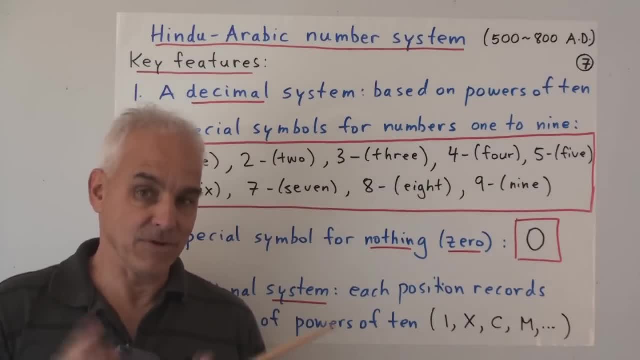 And five by three was 15, was odd, and so there were no ways of tiling this. So the answer to our counting problem was zero, nothing. There are no ways, So this is a possible answer to a counting problem. It could easily be that you're trying to count something. 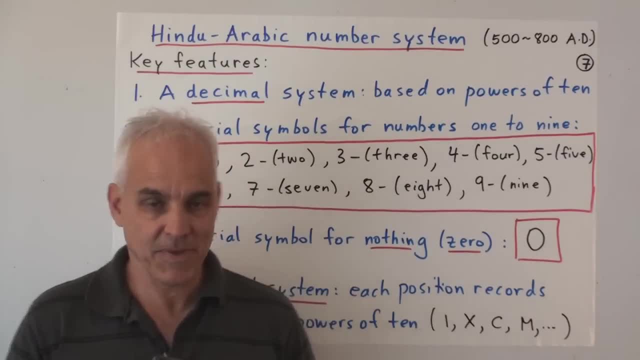 you get zero. That's a very possible answer. With the Hindu-Arabic system, we now have something that we can write down on the page representing nothing, Not just blank. This is very important because it feeds into this fourth key point. 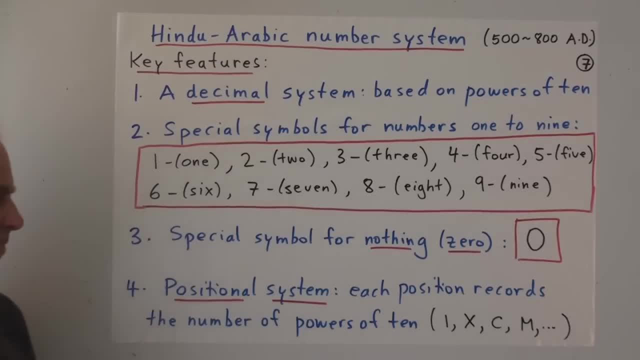 That the system is going to be a positional system. We're going to write down a bunch of these symbols, from one to nine. They're each going to be in a position which records a certain number, A certain power of ten. So we're not going to use these Roman numerals anymore. 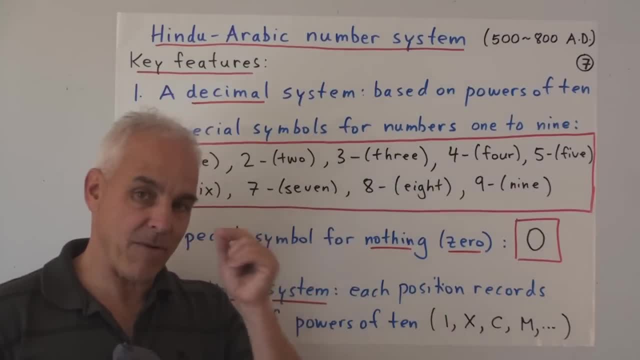 but nevertheless, the idea of the Roman numerals is going to be in the back of our minds when we move to this Hindu-Arabic system. So let's see: how does this actually work in practice? How do we actually write down the Hindu-Arabic form? 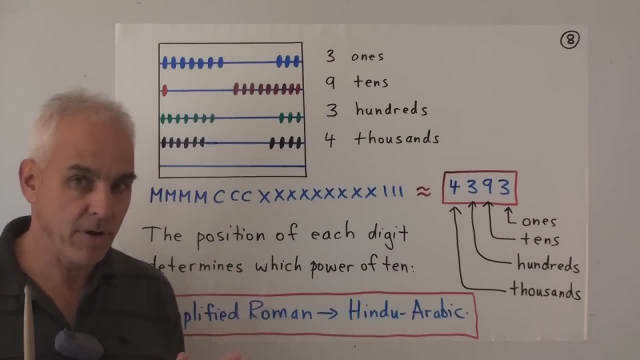 for a number. Well, let's start with a number on an abacus. This number right here. So we've slid over a certain number of blues, a certain number of reds, a certain number of greens, a certain number of blacks. 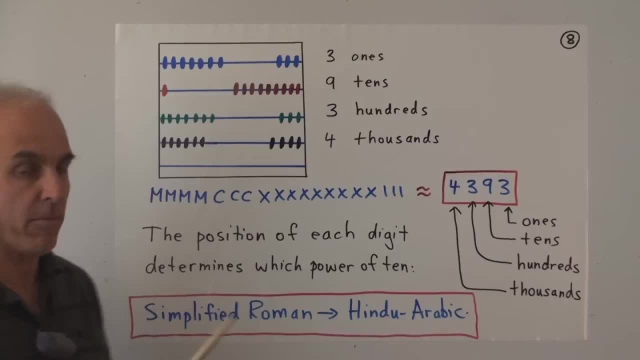 and the number that we've slid over here on the right hand side represents our number. We can count that we have three ones, we have nine tens, we have three hundreds and we have four thousands. So in Roman form, or in simplified Roman form, 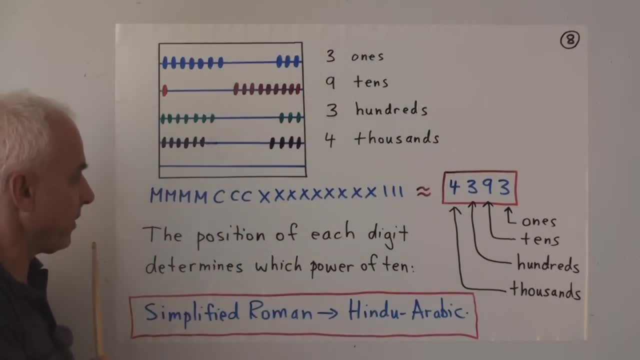 we would write this number down in the following way: We would write it by first starting with the thousands and writing an M for each of these thousands. So M, M, M, M, And then the hundreds C, C, C. 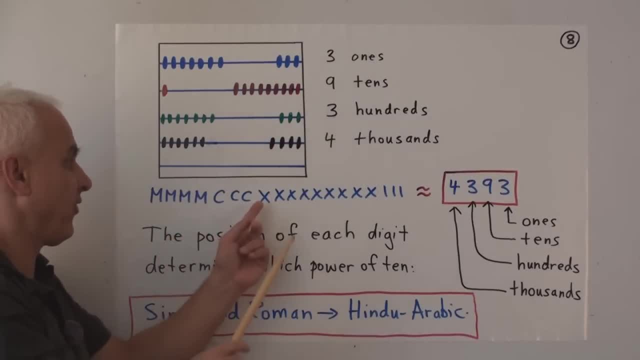 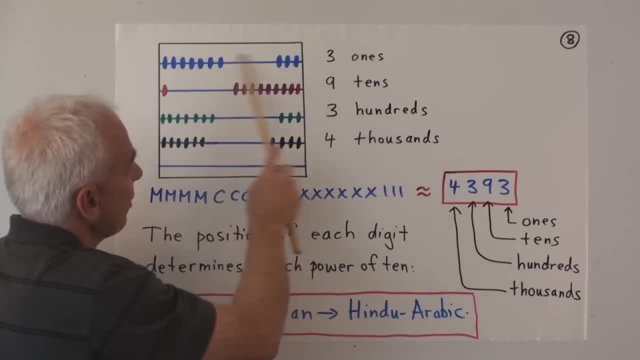 So this line here represents three ones, because this we've agreed that everything on this bar is a one. Here we have nine tens, because everything on this bar is a ten. Here we have three hundreds, because everything on this bar is a hundred, And here we have four thousands. 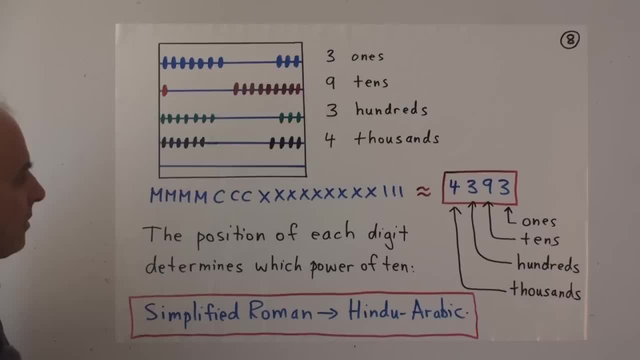 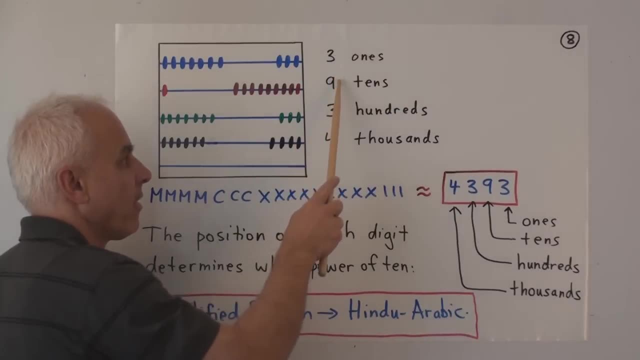 because everything on this bar is a thousand. And now what we're going to do is we're going to write down these numbers, And we're going to write them down from right to left Or, if you like, we can read them up like this: 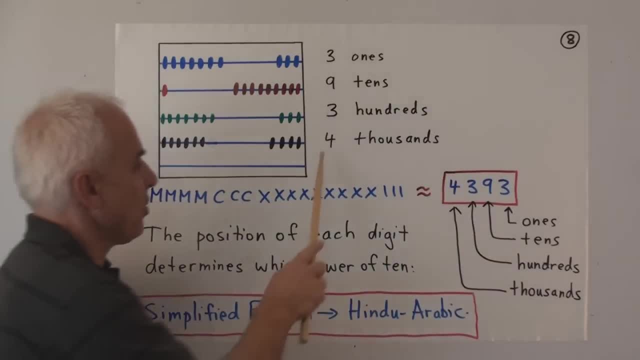 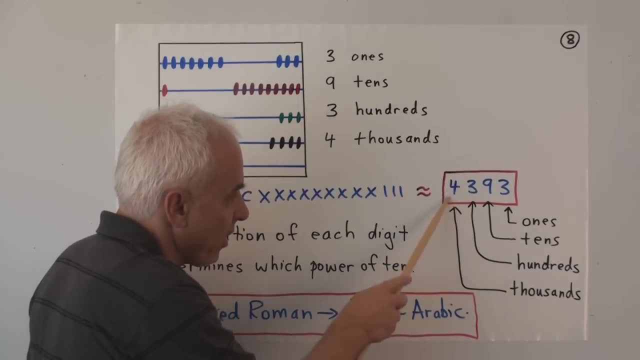 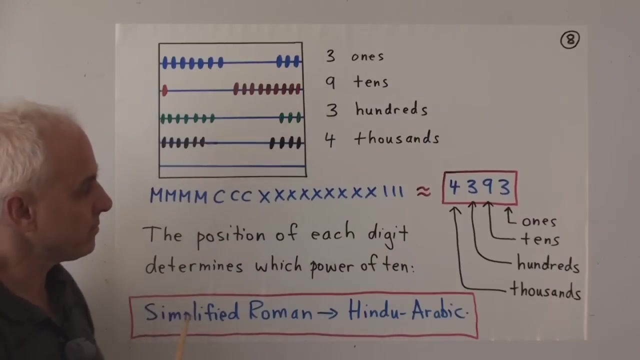 and then write from left to right: So four there, three there, nine there, three there, And what is it telling us? It's telling us that there's four thousands. So this four is in the thousands place, just like this four here was in the thousands row. 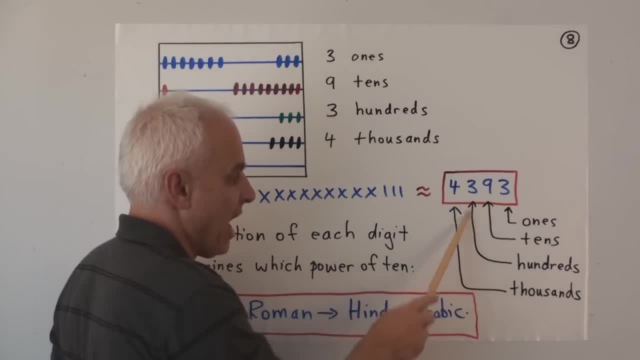 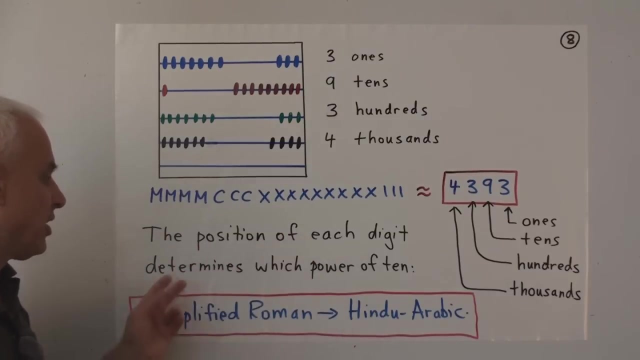 So we have four thousands, We have three hundreds. That's in the hundreds place. We have nine tens And we have three ones. That's what we mean by. it's a positional system, So the position of each digit determines which power of ten we're talking about. 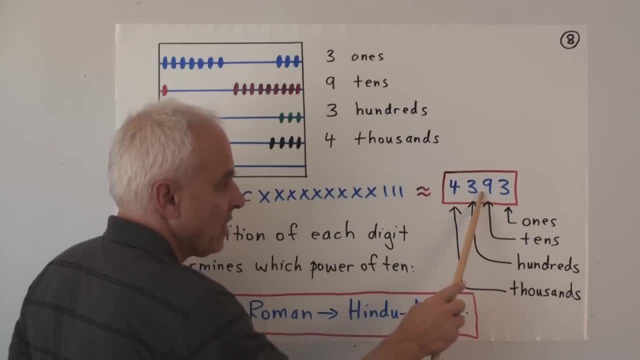 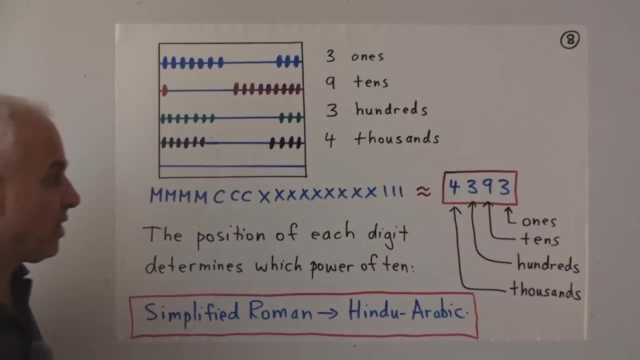 This is the ones position, This is the tens position, the hundreds position, the thousands position, And if we kept on going and we had more bars, well, we could add further numbers to the left representing larger and larger units. So here is this point that I'm trying to make. 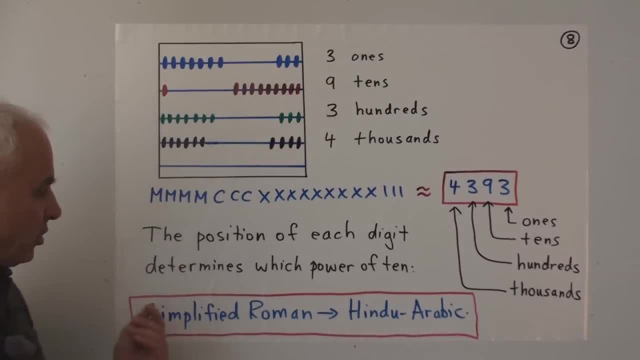 that it's a lot easier, I think, to learn Hindu-Arabic numerals as a modification of the simplified Roman system. You can see that if you were working with numbers like this a lot at some point you might have the idea. you might say: 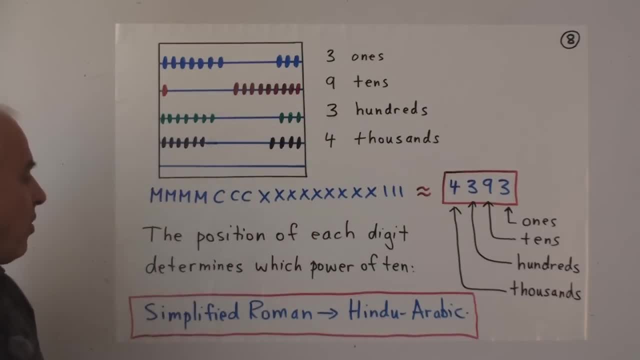 look, this is a waste of time having to write down all these things. Why don't we just record how many ones we write, how many x's we write, how many c's we write and how many m's we write, Because we can use our symbols. 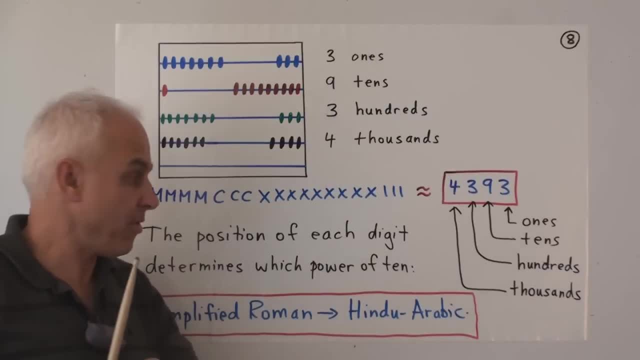 for one to nine to record each of those numbers. So in other words, the symbols from one to nine are not just being used to count ones, They are also being used- a little bit more flexibly here- to count how many tens there are. 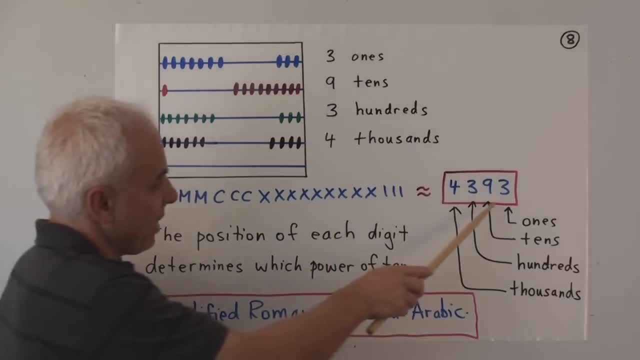 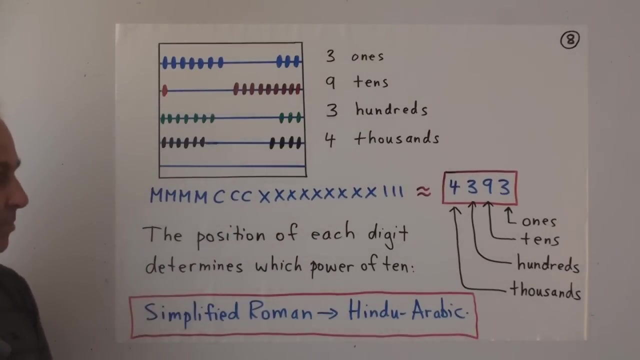 or how many hundreds there are, or how many thousands there are, and that's what ends up in the various places. So my guess is that students and learners benefit by first working a little bit with this simplified Roman system and then realize that the Hindu-Arabic system 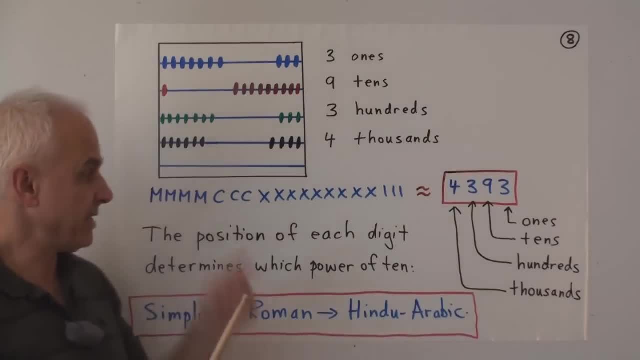 is a step up from this one. It's an improvement on this. Somebody had a good idea. Going from here to here is a good idea. It's a very, very good idea. You might say, oh, I would have thought about that too. 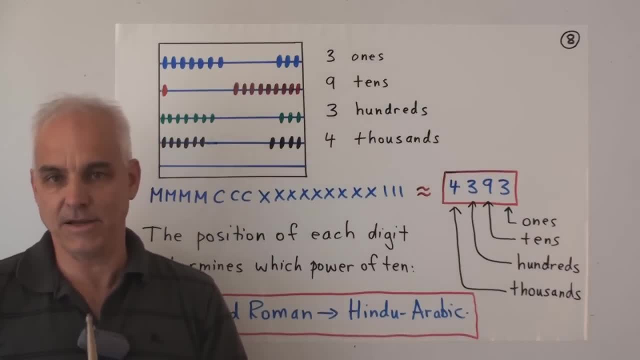 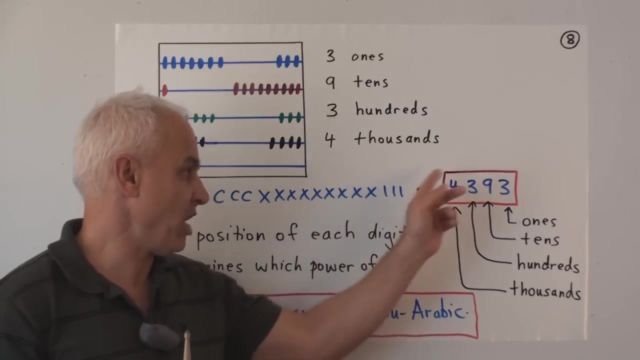 And maybe we should have that idea. After all, we said, mathematics is common sense, But this is a great piece of common sense here that no previous culture was able to make this jump. It's a very big jump going from this level to this level. 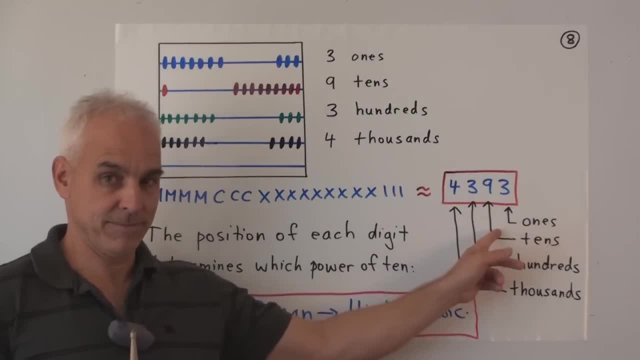 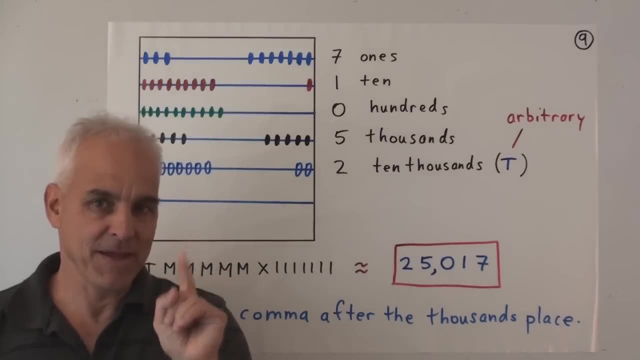 Basically from the ancient world to the modern world. It's that big a jump. Now I still have to explain the importance of this zero. It's crucial for this system that we have a zero. Let's illustrate that with this second example here. 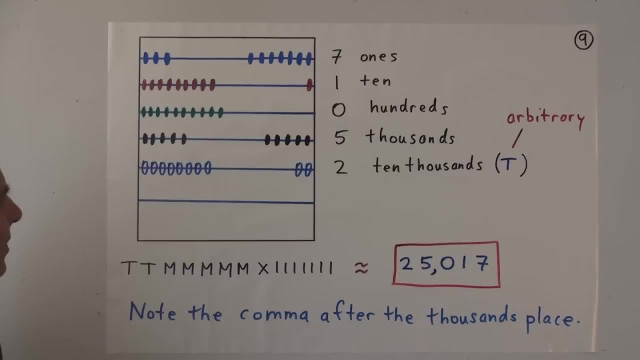 So we have another number recorded on the abacus. This time we've got How many are over here. By the way, I can figure out how many there are over here by noticing that there are three over here. I know that if there's three on that side. 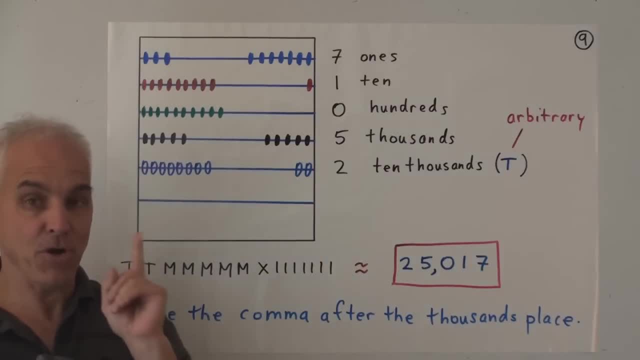 there's going to be seven on that side. It's one of the things that you learn by playing with an abacus. It's actually a very important thing to learn That three on this side means seven on this side, If there's one on this side. 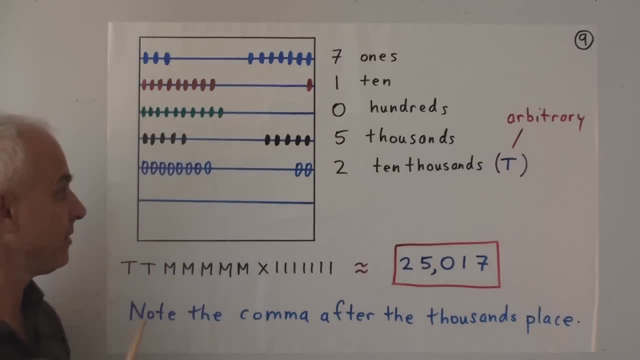 how many are there on this side? Nine. If there's five on this side, how many are on this side? Five. So you learn to match five with five, Four with six, Three with seven, Two with eight, One with nine. 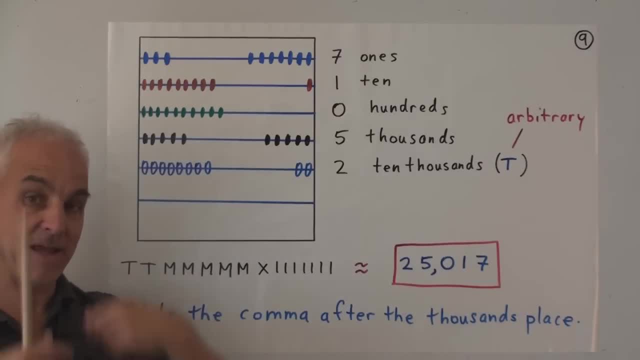 Those are very important matchings. They match up, They add up to ten. So we see that there are seven ones moved over, There's one, ten moved over, There's Well, there's no hundreds moved over. All ten hundreds are still over here. 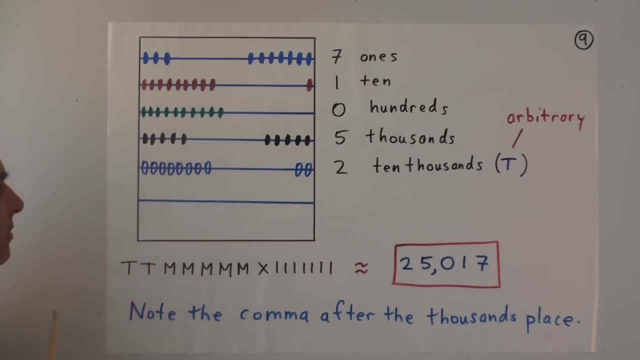 on the left-hand side. Okay, Then there are five thousands moved over, And it looks like we've moved down a level. We've got even a bigger number. We've got some new kind of unit, of which there's two of them. 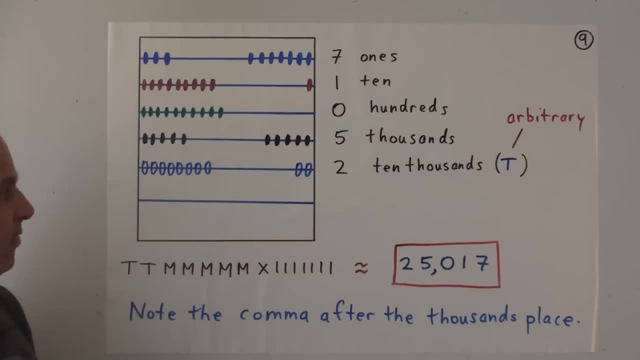 And these units should be ten times as big as the previous ones, So they should be ten times a thousand. Well, we don't have a new name for those units. We could, but the standard thing is just to call them ten thousands. 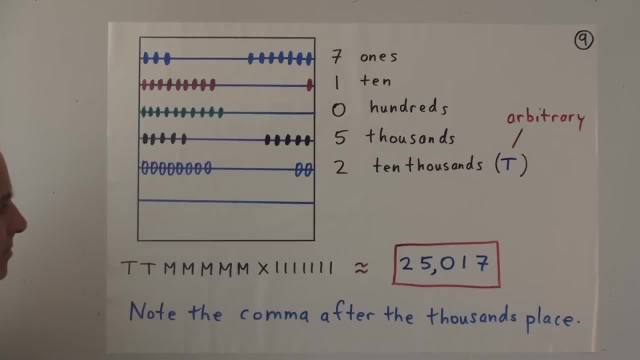 So we have two ten thousands Now. the Romans didn't have a symbol for ten thousands, but we would like to have a symbol for ten thousands, And so we're going to augment our Roman system a little bit and allow me to introduce T for ten thousand. 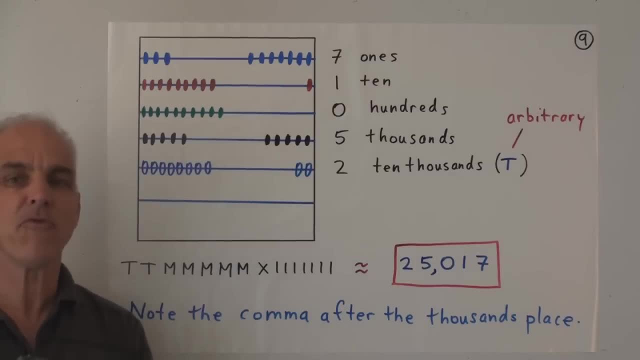 Okay, There's a long overdue improvement on the Roman system. We're now going to add T, so that means we can talk about bigger numbers than the Romans used to, So this number that we've recorded here in Roman form would be well. we start with the biggest ones. 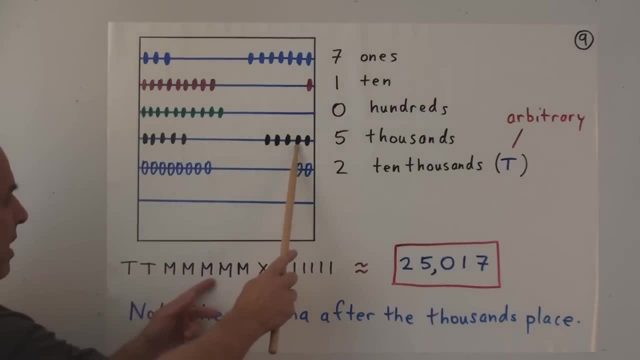 T, T, And then M, M, M, M, M. And then, well, there's no C, so we wouldn't write down anything. We would go to the tens. There's one ten, And then there are seven ones. 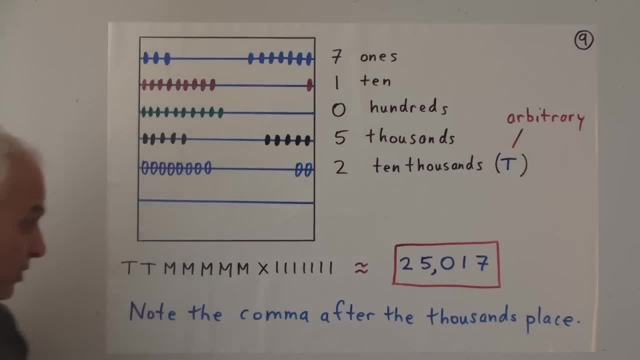 So we make no mention of that number. That's the fact that there aren't any C's. You can see that there are no C's. because you can't see any of them, There's no need to draw special attention to them. However, when we go to the Hindu-Arabic system, 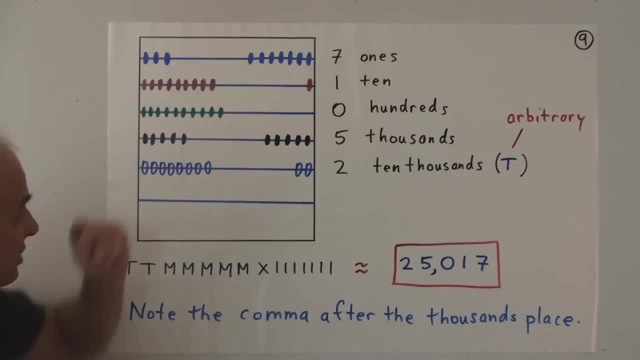 things are different Because in the Hindu-Arabic system every line counts. We have to record what's on every line. Just because there isn't anything on a line doesn't allow you to ignore that line. We still have to put something down. 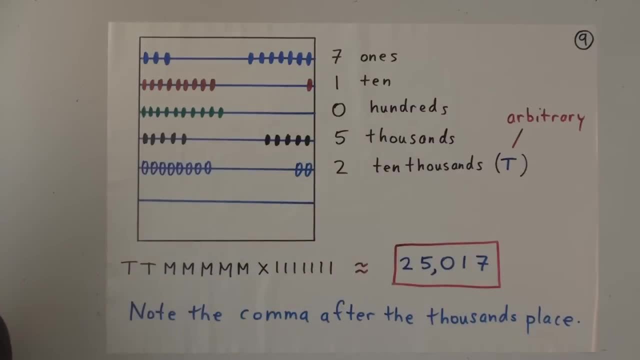 And that's where the zero comes in. There are zero hundreds Because we have a symbol for zero, A new symbol That essentially none of the ancient cultures had. So we have seven ones, one ten zero hundreds five thousands and two of these new ten thousands. 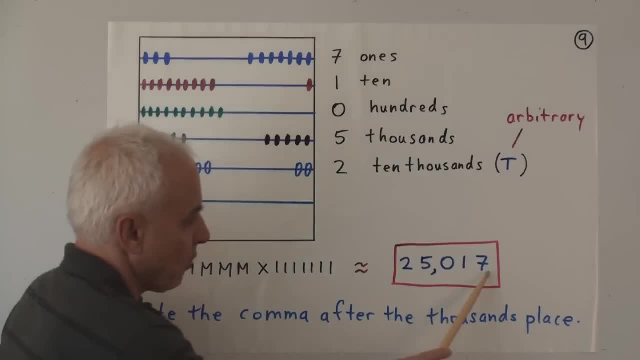 And we're going to string them all together, Starting with the ones on the right-hand side: Two ones, one ten zero hundreds five thousands, two ten thousands. Or, if we had started from the Roman number, we could start either from the right or the left. 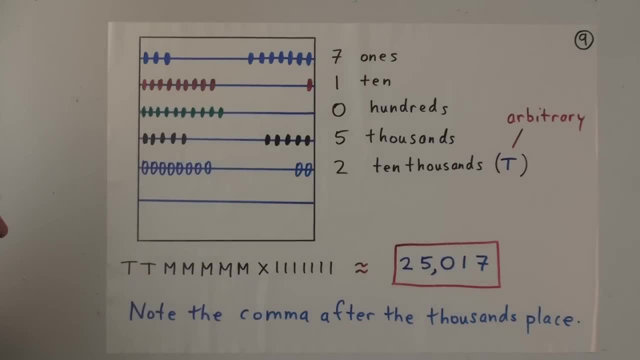 Let's start from the left, sort of more in keeping with the spirit of things. So the two T's would be two, two, ten thousands and then five thousands zero hundreds. There aren't any hundreds, but we have to record that. 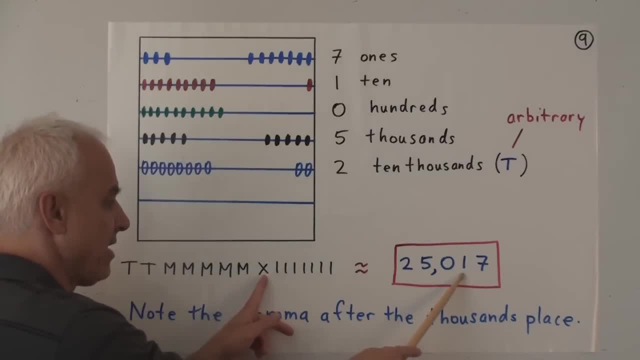 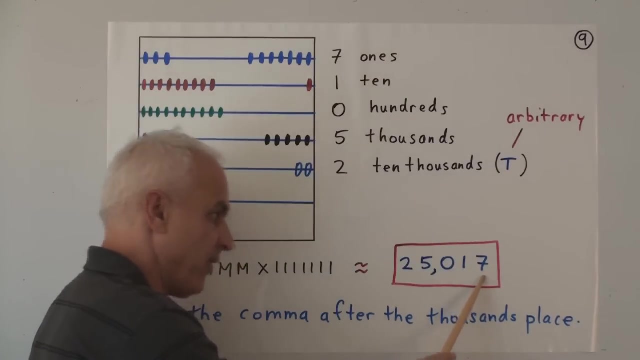 Because this is the hundreds, position One, ten and seven ones, To see what position it is. it's often a little bit easier to start from the right, Because then you're guaranteed that you're going in the right direction. We can say: that's the ones. 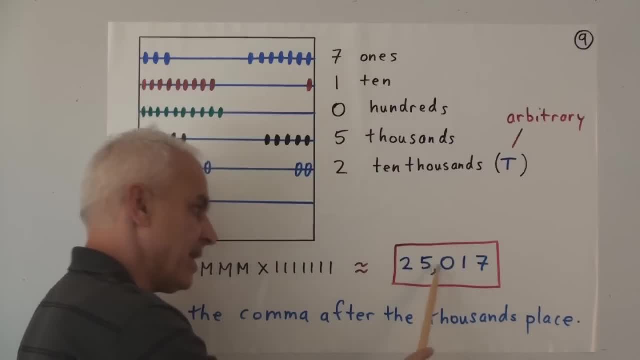 that's the tens, that's the hundreds, that's the thousands, that's the ten thousands. You know you're in the right spot because every time you're going up by ten And note that we're introducing a small convention, We're putting a comma right here. 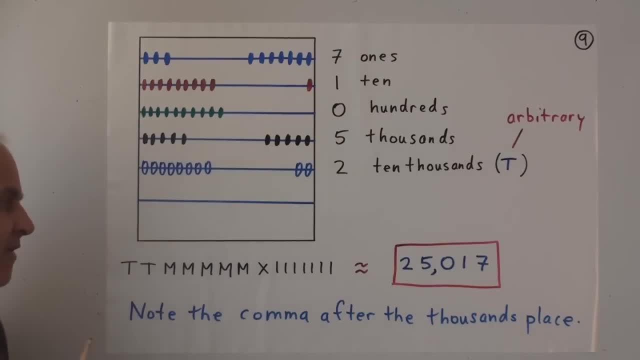 That's just a little bit of a helpful device to make it a little bit easier to see where things are. So we put the comma after the first three digits representing the ones, tens and hundreds. So after the hundreds there's a comma before we get to the thousands. 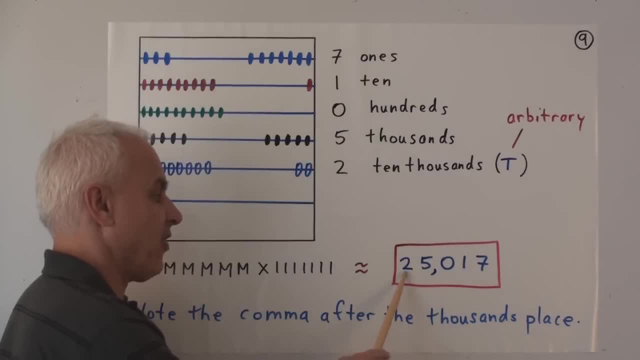 And we would write this, we would say this as twenty-five thousand and seventeen. We'll talk about the names for numbers later on. Right now, we're just going to write down this number. That's our Hindu-Arabic form for this Roman number. 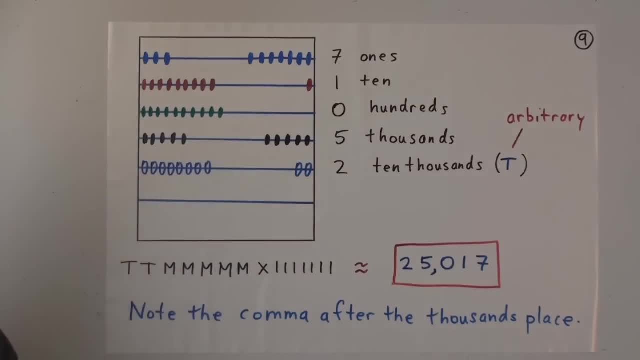 or this Abacus number. Now I think we can be reasonably sure that the Hindus who first developed this system were probably thinking more in terms of an Abacus than they were some other system. They had some Abacus, they had some counting frame. 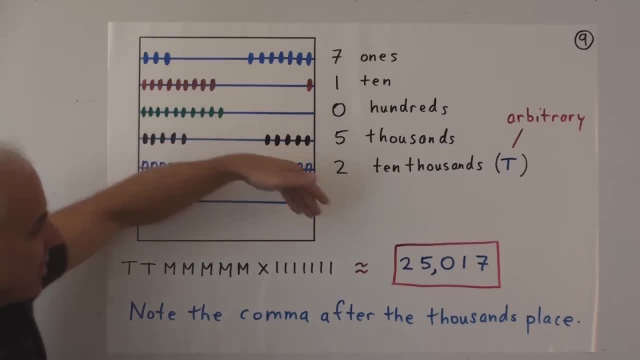 they wanted to represent what was going on there. that number compactly And it makes a lot of sense just to record how many there are in each row. So from a counting frame or Abacus point of view, the Hindu system is very natural. 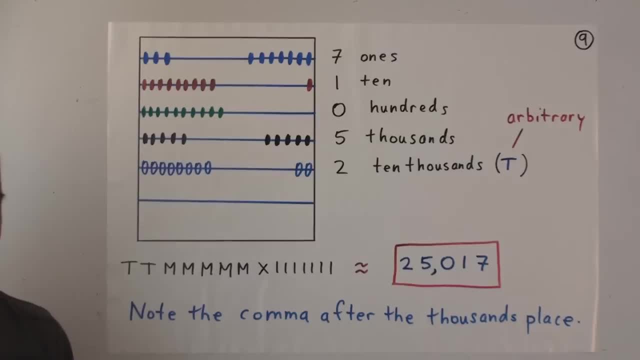 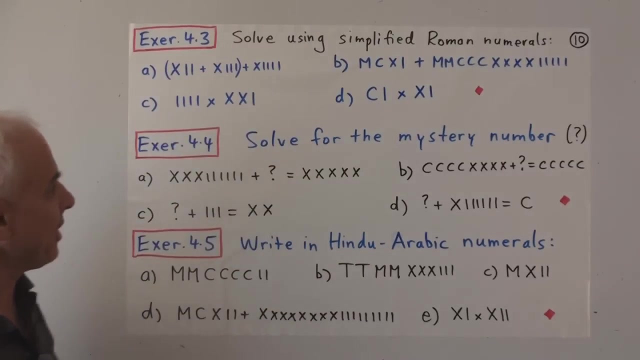 Okay, so that's good. We've introduced our basic number system that we're going to be working a lot with in this course. So now it's time for a few exercises for you. So exercise 4.3,: solve these arithmetical problems. 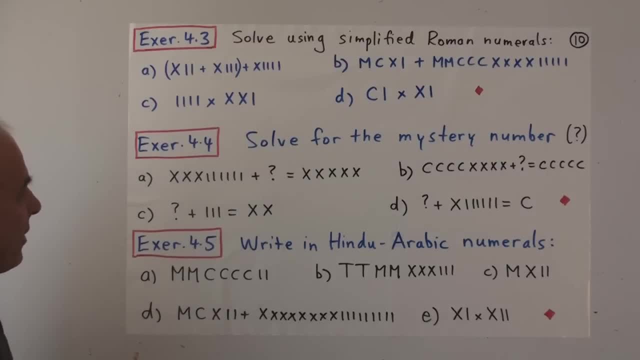 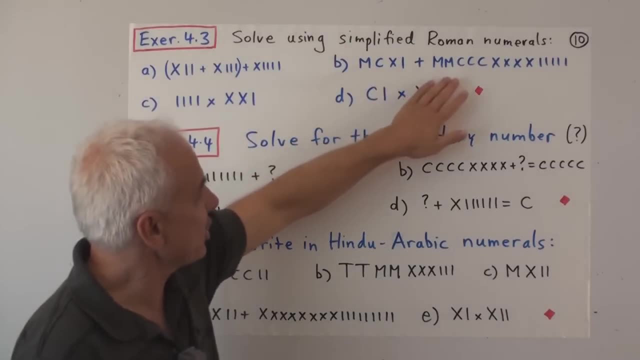 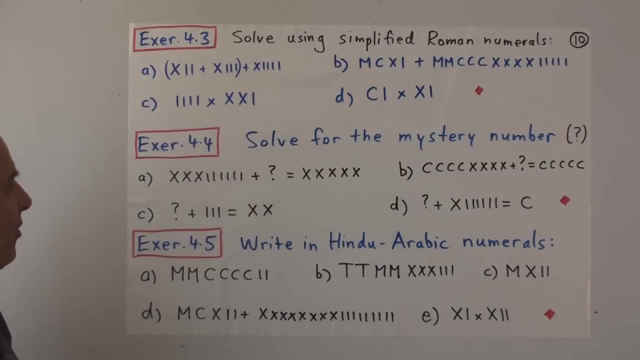 in the framework of the simplified Roman numerals. So here's an addition question with actually three things being added. Here's an addition question with some bigger numbers. Here's a somewhat smallish multiplication- not too small, though- And here's a kind of a bigger multiplication. 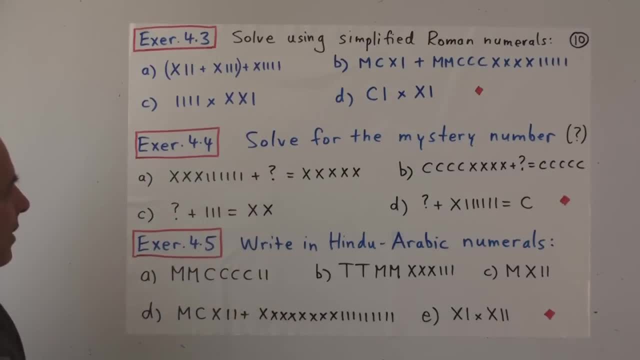 because that's a hundred there. So in each case, I want you to think about: what does it mean? what do these questions mean geometrically, in terms of rectangles? Can we figure out what the answers are Just using geometrical intuition, maybe drawing some diagrams? 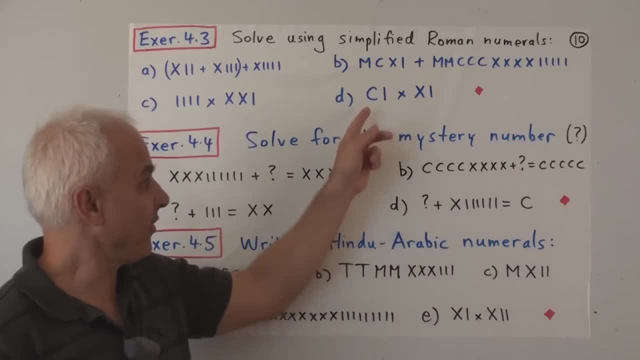 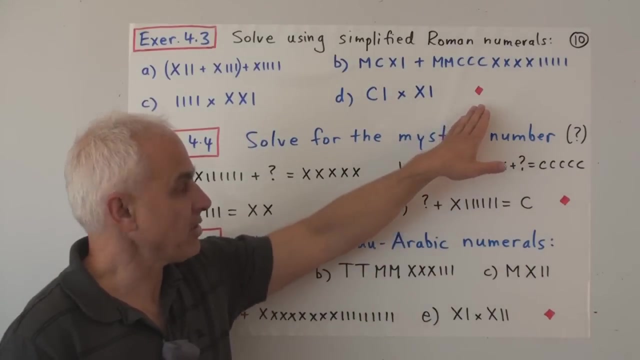 This one. here you may have to do some lateral thinking, because this rectangle here would have 101 rows and 11 columns. It would be pretty big to draw. So you might think, well, is there some snappy way of doing that? I want to get across to you that multiplication. 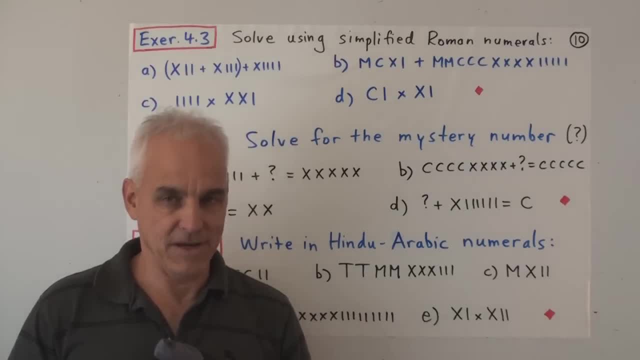 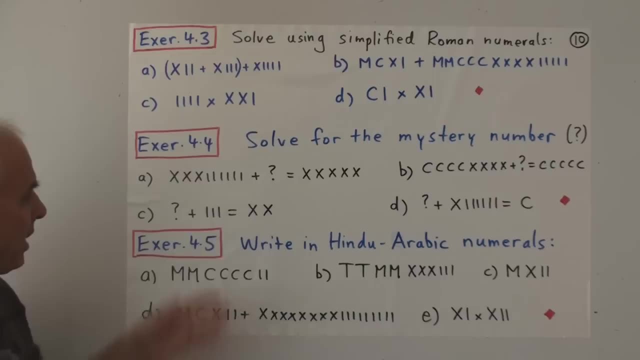 is quite a lot more difficult than addition. So we're going to see that major theme in K-6 mathematics In this question. here we're solving for a mystery number represented by a question mark. So this number plus some mystery number is this number. 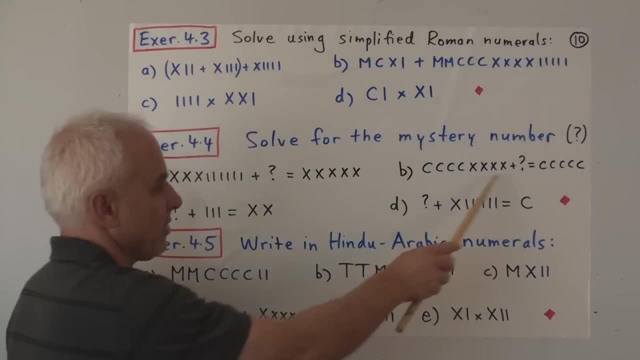 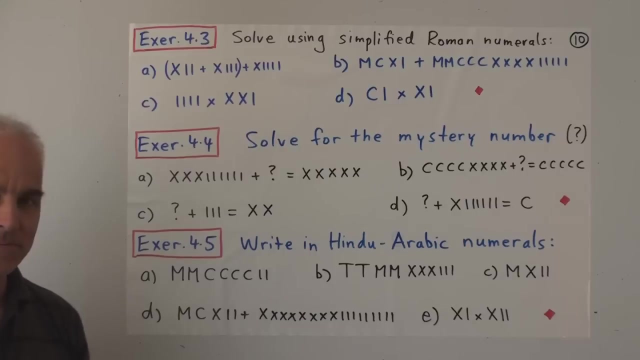 And you're supposed to try to figure out what the mystery number is. Here's another one. Here's mystery number plus 3 equals 1010.. And mystery number plus this equals 100.. And our last exercise, just to convert these into Hindu-Arabic numerals. 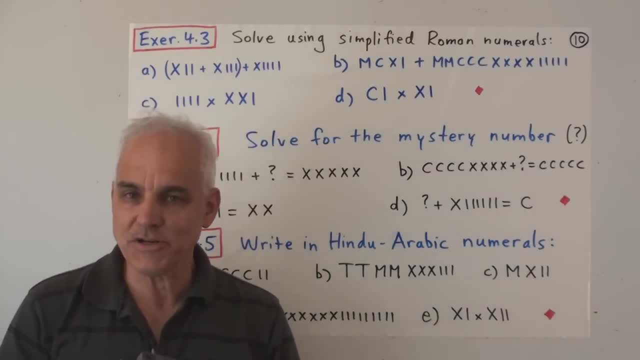 Now that we have at least some terminology, we can now use our Hindu-Arabic numerals. I don't have to keep saying 1,, 1,, 1.. I can talk about, you know, 12 and 13 a little bit. 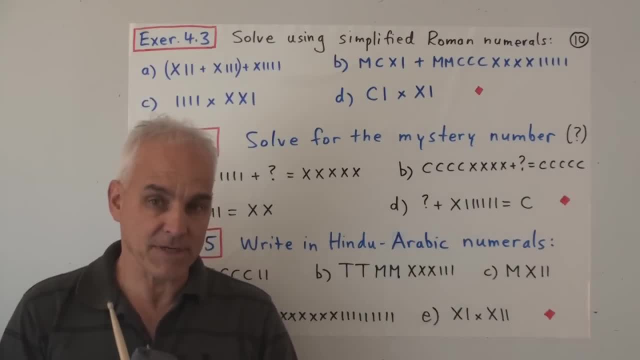 We're going to go back to the basic laws of arithmetic now And we want to understand the laws of arithmetic from a geometrical point of view. So we're going to go back almost to this kindergarten approach and now ask ourselves: well, how does one actually, you know, 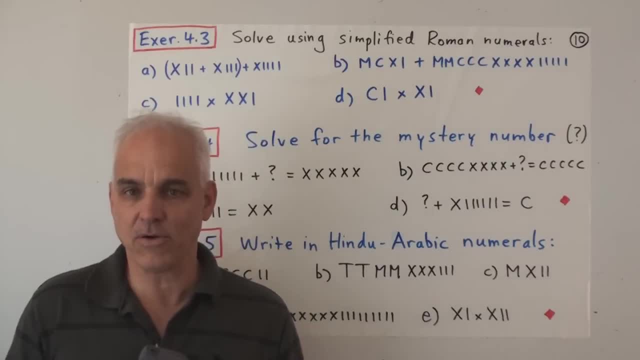 how does one actually multiply? How does one actually add? How do we figure out efficient ways of doing that? That kind of question is best addressed by going back to the more primitive kindergarten form of numbers as row rectangles. So I hope you'll join me for that. 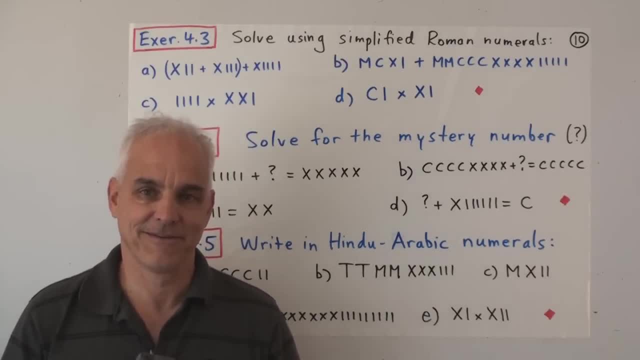 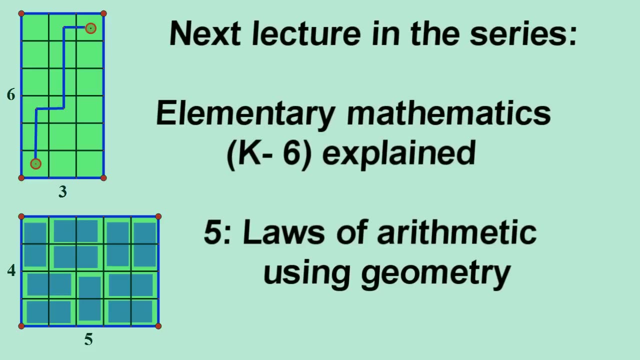 I'm Norman Walburger. Thanks for listening.